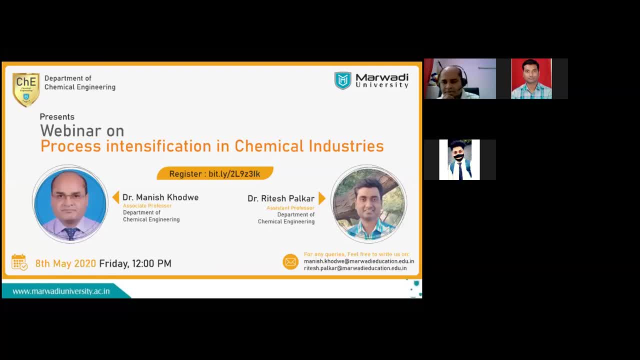 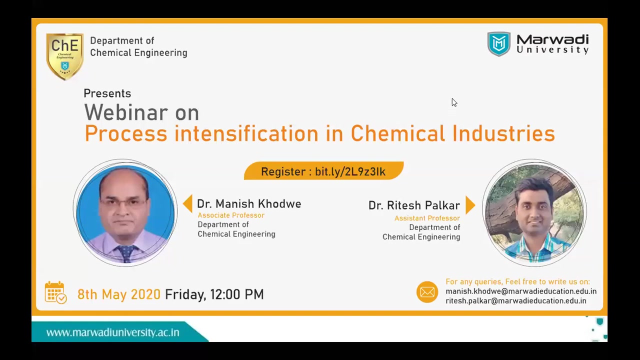 Good afternoon everyone. I'm Dr Ritesh Palkar, working as Assistant Professor in the Department of Chemical Engineering Faculty of Technology, Marwad University. Welcome you all on this second webinar which we are conducting on Process Intensification in Chemical Industries. 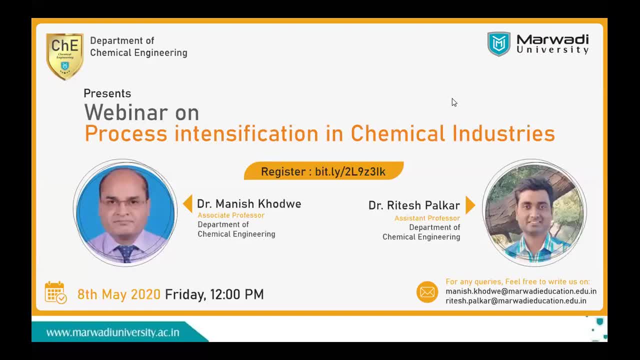 I know there are many participants, those who are joined to us. They are from different backgrounds apart from chemical engineering. But here we are going. we are planning to discuss about basics and somewhat principal applications of Process Intensification. So I welcome my co-host, Dr Manish Khodway. He is working on Process Intensification in Chemical 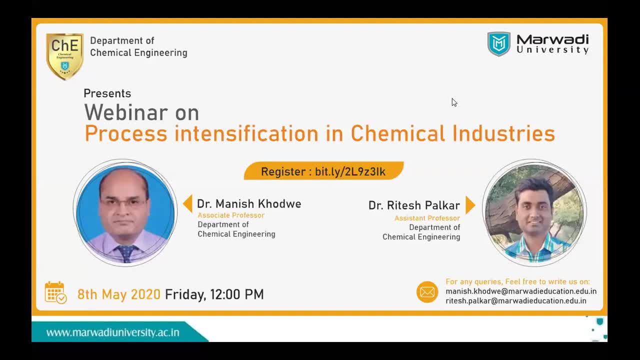 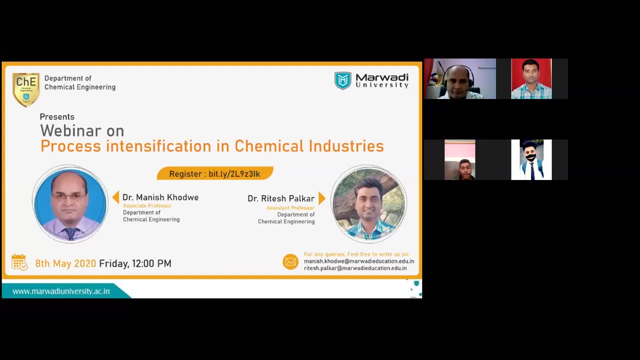 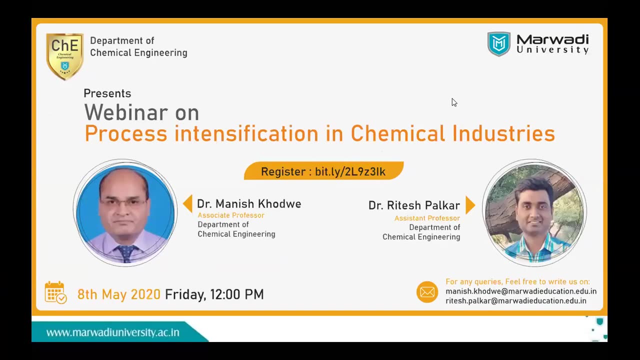 Industries. He is working as Associate Professor in our Department of Chemical Engineering. He is having 20 plus years of experience in academics as well as in industry. So today we are going to discuss about Process Intensification in Chemical Industries. Okay, So let us start. 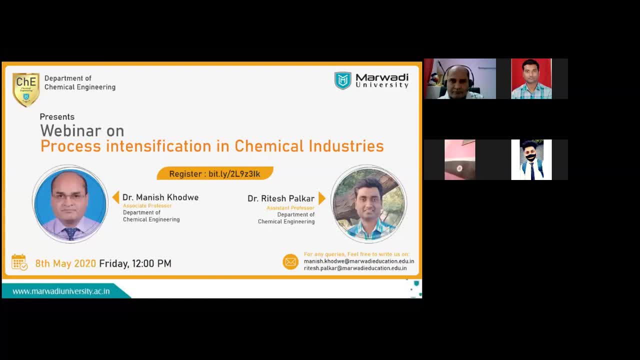 In meanwhile, if some students, those who will come in between, we will try to, we will try to accommodate them in between. Okay, So we'll start with this. Manish sir, are you audible? Yes sir, Yes sir. 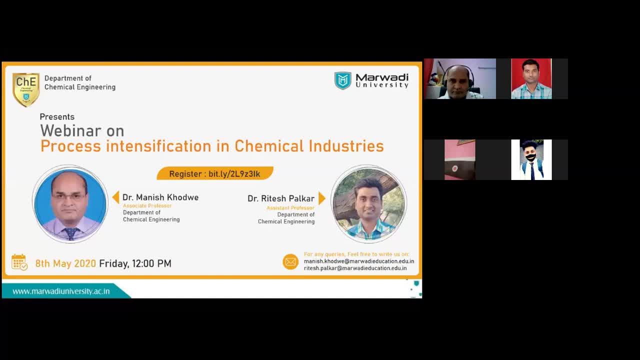 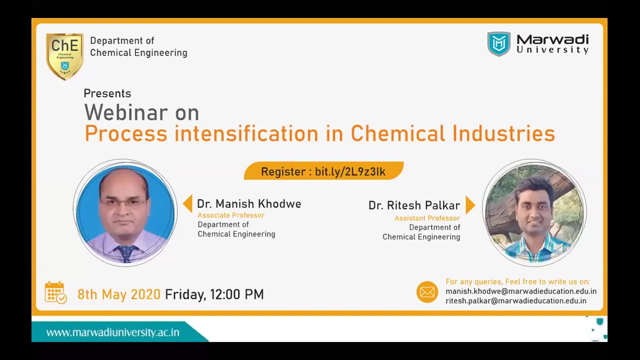 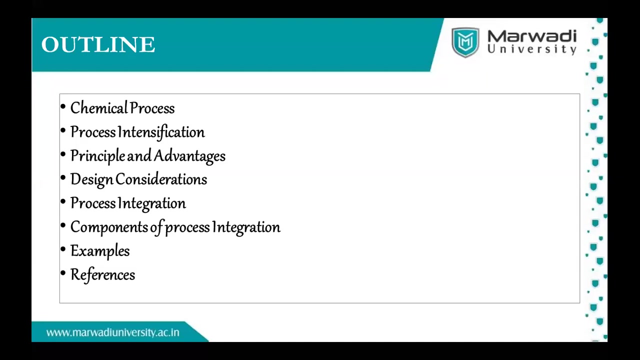 Yeah, So we'll start with the outline of today's discussion. So today we are going to discuss about second slide, please. Yeah, today we are going to discuss- we'll start with the in general. what is chemical process? how the changes are occurring inside the system that we are going to discuss as 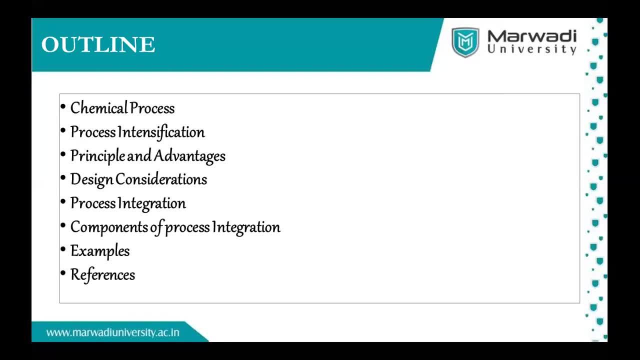 a preamble of this today's talk. Second, very important: What is Process Intensification? Okay, What are the pro and cons of present systems And how the Process Intensification has come into picture in today's life? Next, What? 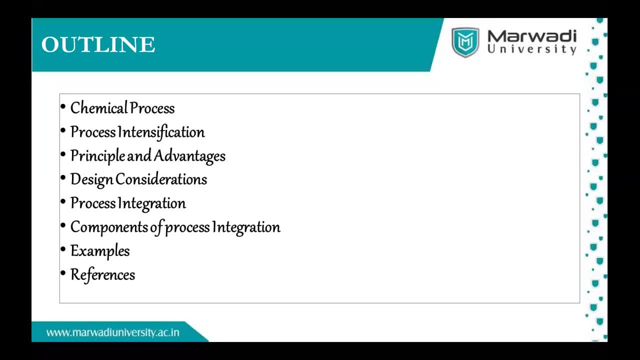 are the principles and advantages. Apart from that, there are different kinds of theories available for Process Intensification. So for this we will try to discuss different kinds of principles as a part of basic discussion, basic study, and what are its advantages simultaneously. 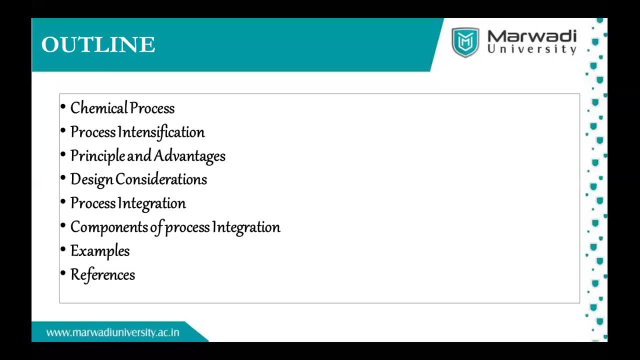 As a chemical engineer, we have to deal with a different kind of design parameters. So the fourth point which we are going to discuss today is about what are the design considerations when you guys will go for process intensification. Next, as we will discuss first point as chemical process, so how to do the integration of all 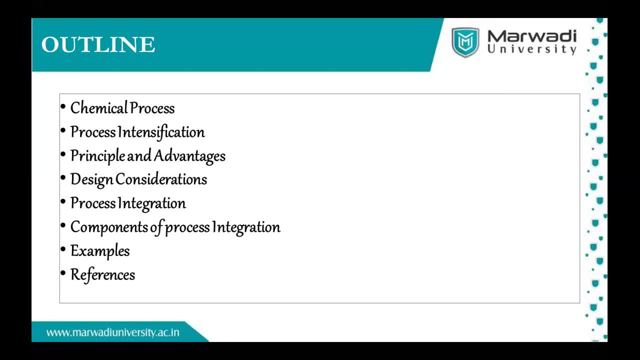 these processes will be discussed by me and Dr Manish Khodve, And if we are discussing about the process- intensification and how to do the integration, so what will be its component? that is also an important discussion which is to be had. 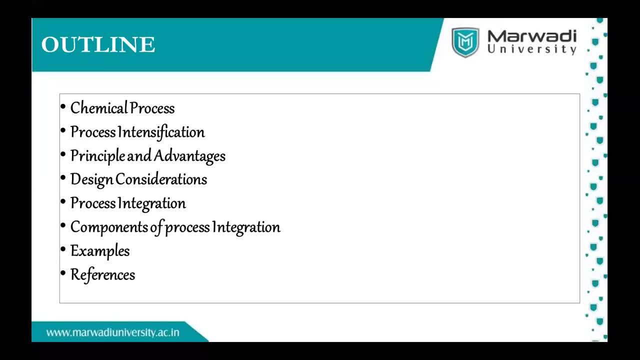 and highlighted, I feel, in due course of time. So at the end we will try to show you some kind of examples which mostly referred as one of the reference basis for process intensification. So, as you may aware about that, process intensification has recently started. 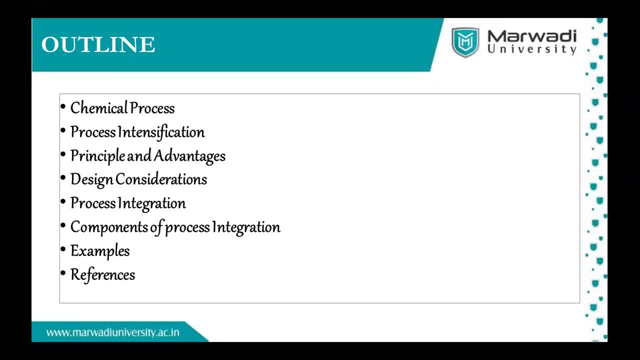 In 1990s, in one of the conference, this topic was first discussed by Ranshaw and he has given different kind of definitions. So according to that, this is our outline and our aim is by the end of this webinar. 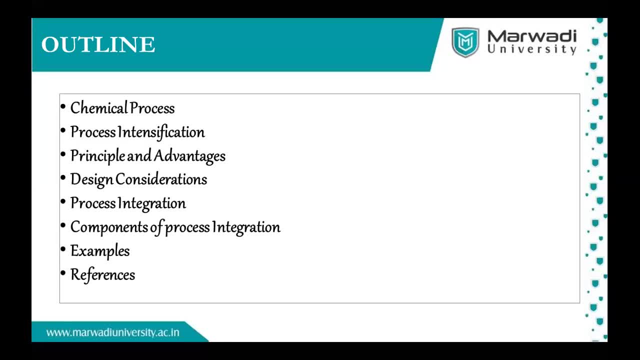 our participants will be able to know about what is process intensification. Participants will be able to identify the process or processes So they will be able to apply the different process intensification techniques and identify and discuss or design the process integration- process integration along with intensification. 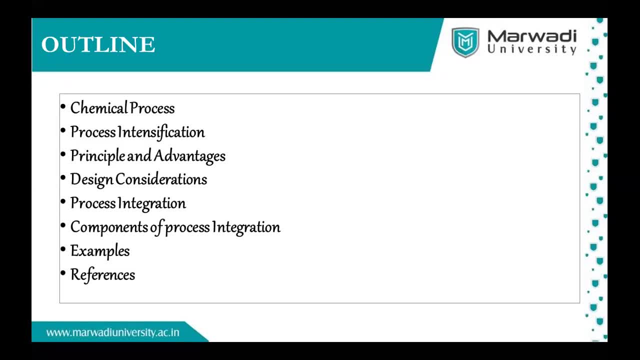 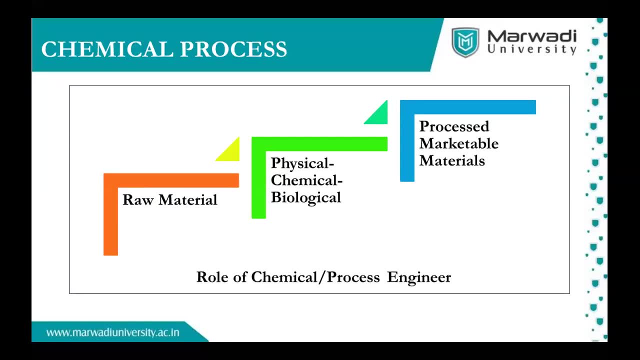 So this is the outline of our today's talk. Next topic is chemical process, which will be discussed by Professor Manish. Good afternoon everybody. Everybody knows about the chemical industry. Normally there are three steps when you are learning the CRE. 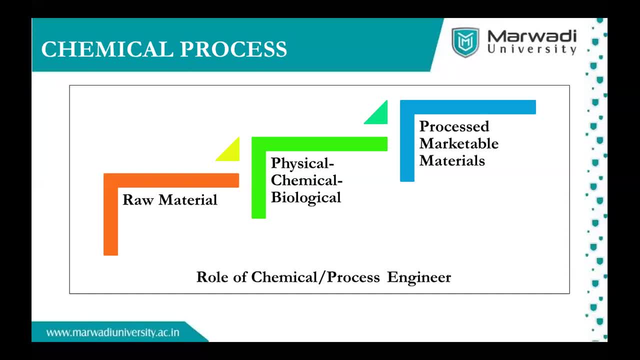 chemical reaction engineering. So these are the three steps. normally we studied, we learned. So the raw material is the first step. normally we require for the processing And the major part is process, whether it is physical or chemical or biological process, And we are focusing on this process. 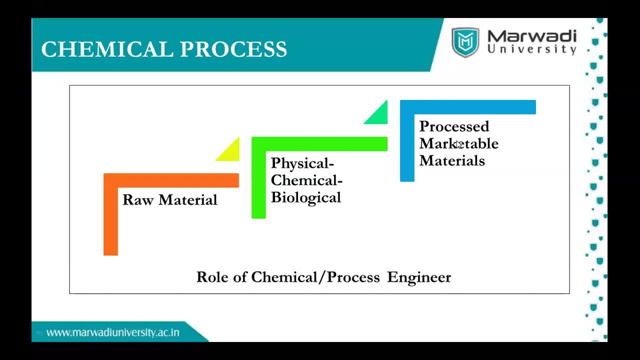 And finally, after this process, we get the product, Which is marketable Means our aim is always to make the marketable. So on that basis, keeping in that mind, we have to do the process which our basic chemical engineering role is there. 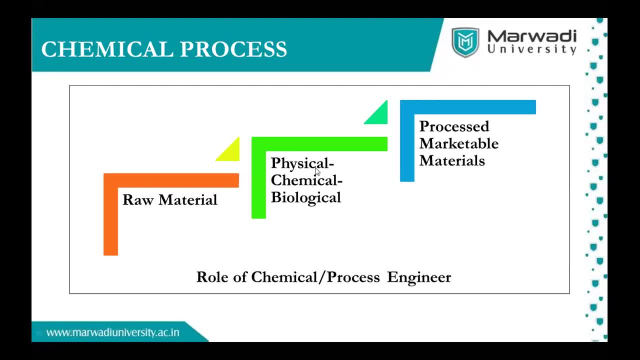 Focus on the chemical process means cost is very, very important. Ultimate aim is the production cost Because the lot of products will be available In the market And we should be competitive. So where we can do the competition, So the major- is raw material. 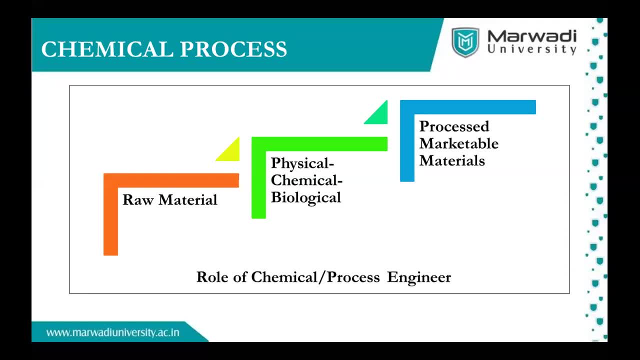 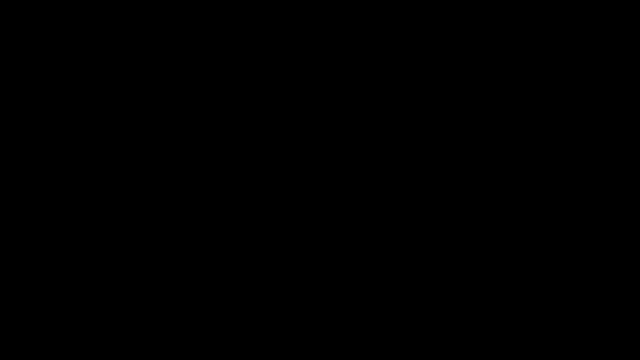 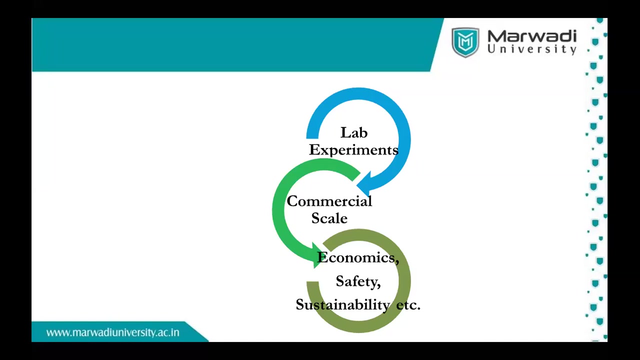 But most of the time the cost of raw material will be fixed And that there is some limitation For the cost of raw material. So we are talking about the chemical process modification, The pressure, temperature and process calculation, Psychometric ratio and all those things. 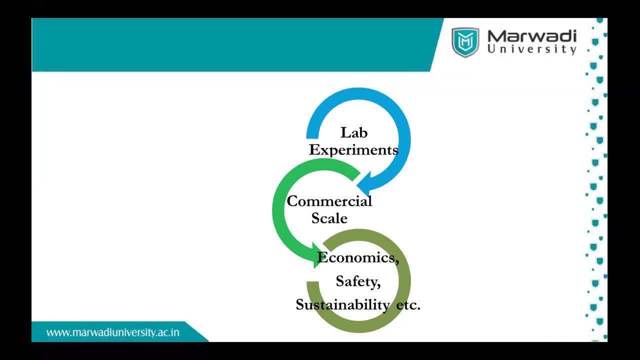 We are optimizing in the pilot scale- That is commercial scale- And then we do the scale up. Scale up means it will be the reaction we are taking in the tons together, or more than that. So normally three steps we are doing in the any industries. 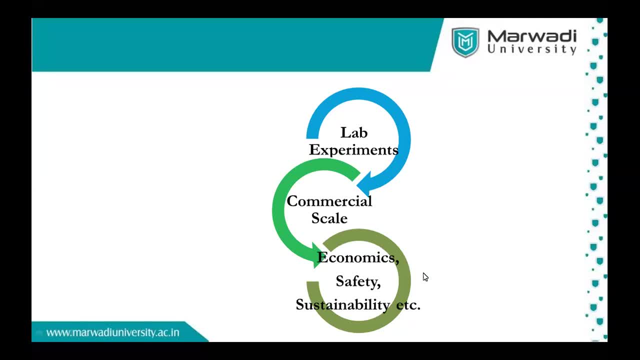 And keeping in mind the economic safety and sustainability. Sustainability means again, We are focused on the Cost. So When we do the modification Or the intense Of any process, We have to Focus On the majorly, The last stage. 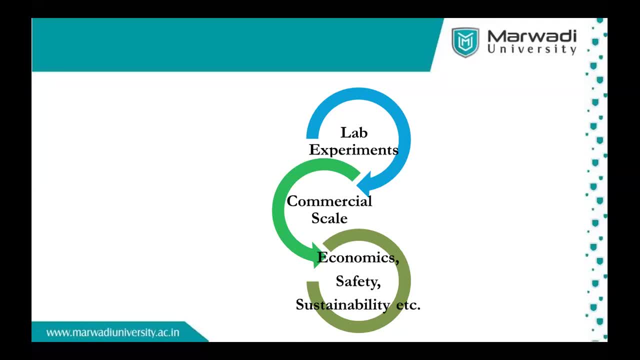 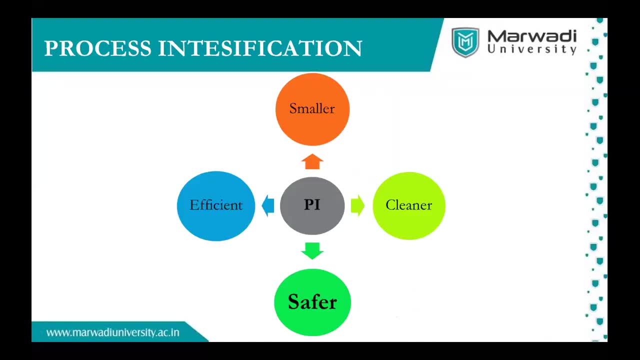 Some do the modification in the, that process In the units And we say it is intensification. So Major objectives of the intensification is The process In the process modification. We want To do the process In that unit. 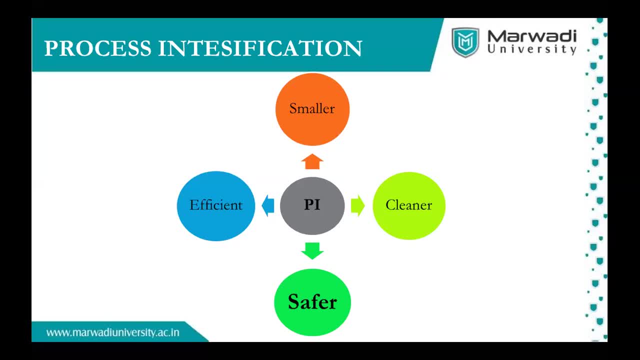 As small as possible, Because you know that When we are Limit tends to zero, Or when we are reducing the size Automatically, the energy Problem Or the Environment problem, Or the handling problem, Everything will be Reduced And automatically. 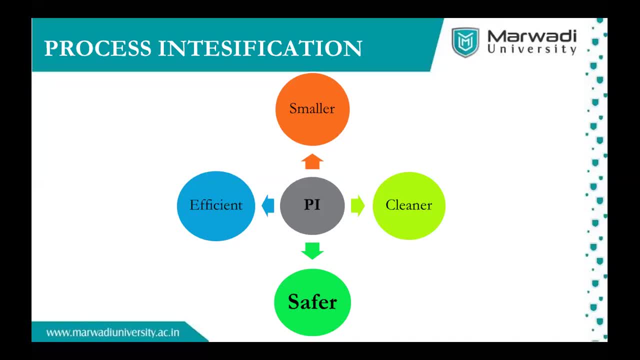 The efficiency Automatically. it will be connected to the That smaller process as well, And definitely When we are reducing the size, We get the Cleaner production also. So Cleaner production, Efficient production And Safer, So Safety automatically. 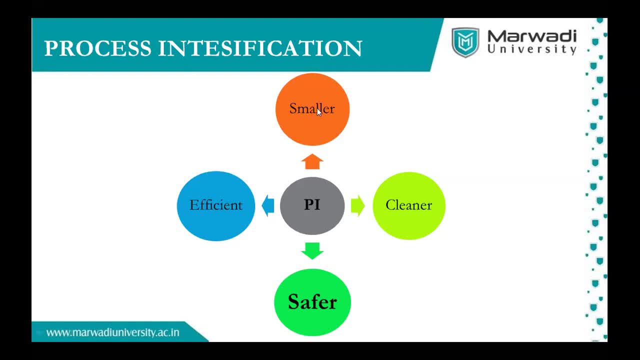 It will come under that. So major is, We have to focus, We have to reduce the size Of that equipment By some modification And We Are Intensification. So If I want to give One small example, 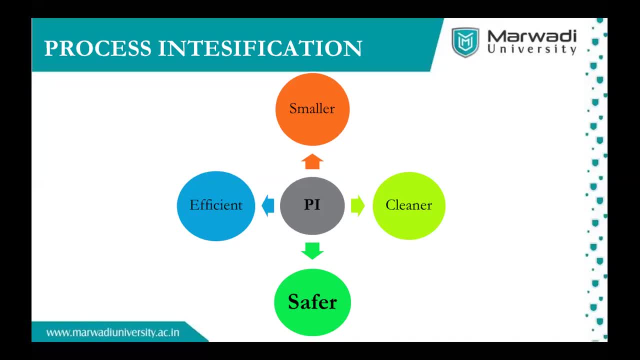 The settling tank Which is coming In the environment Or Influent treatment plant. So If you do The settling By gravity, With the help of Using the gravity Gravitational force, It takes a lot of time. 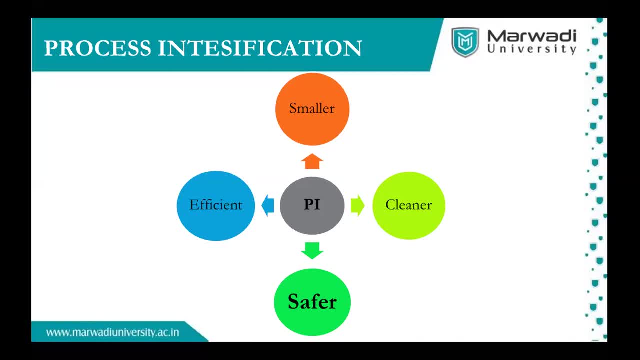 It takes Own time For the settling. So If we use The centrifuge force, If we use The centrifuge, We can do The same Settling Within a short Time. And This is the small. 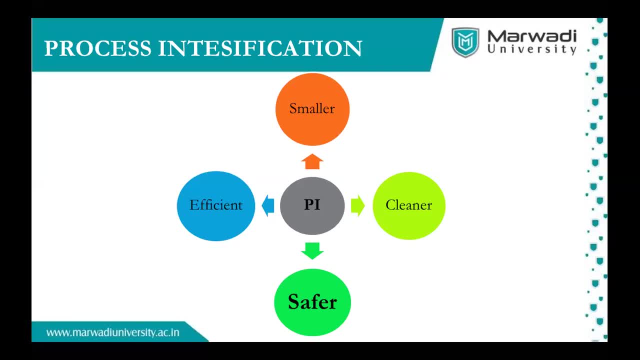 Example Of the Intensification Process. So These are The Small Modification We have To do In Each Equipment. So Ultimately, All Process Intensification As Suggested. 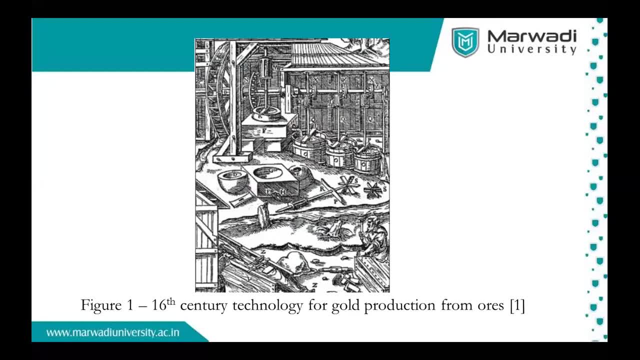 By Dr Manish. It Is A Kind Of Thing Where You Can Improvise Your Process By Considering Those Four Parameters And At The End 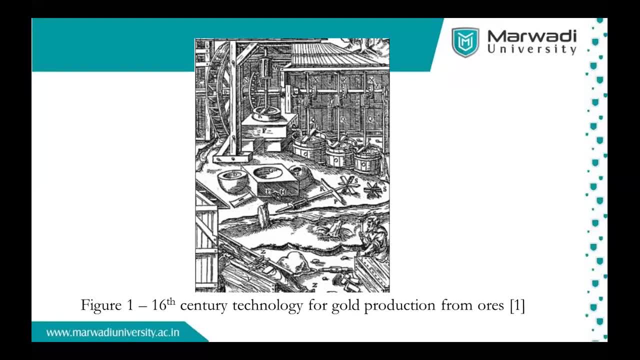 Safety Is From, Let's Say, Starting Of Industrial Revolution. So When You, When You Will Go Through The Different Literature, You Will Be Able To 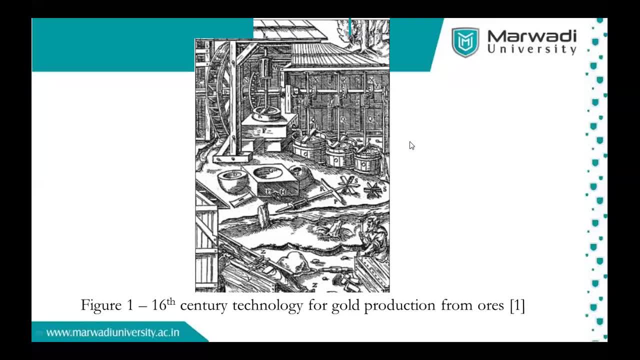 Find Out The Various Examples Based On This Picture Which We Had Kept In Our Slide, In Our On Your Screen. There Are Different Kind. 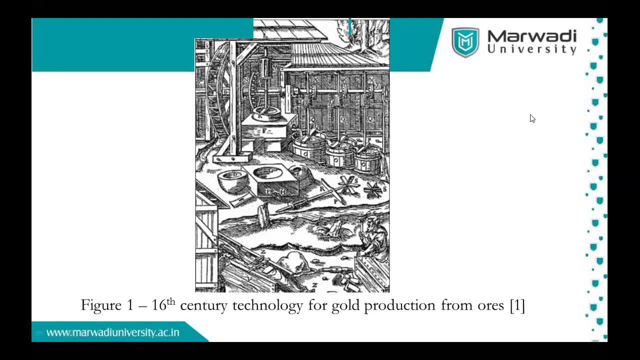 Of Reactors, Stir Tanks, Stores, Right And How These Are. What Are Its Shape Sizes? What Are The Reactors, What Is CSTR, How They? 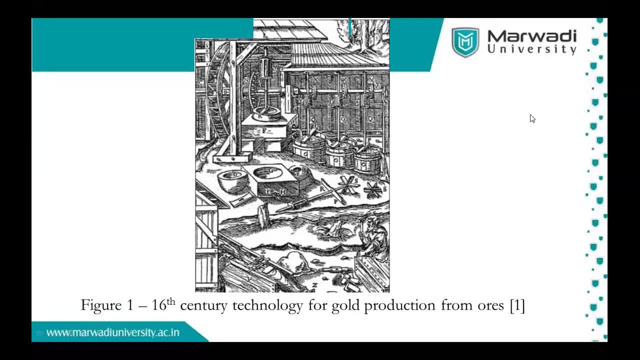 Are Connected In Series Or Parallel, So Different Kind Of Things. You Can See From What We Are Started With, So You Please Do Remember This. 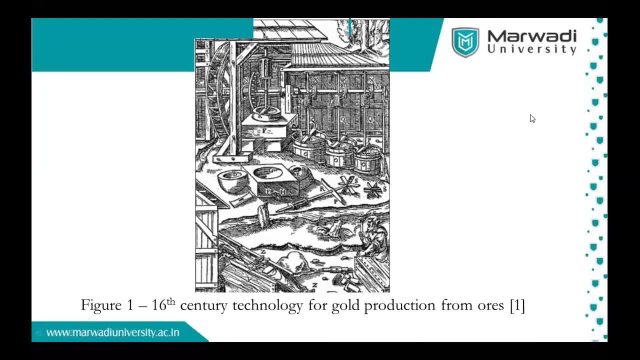 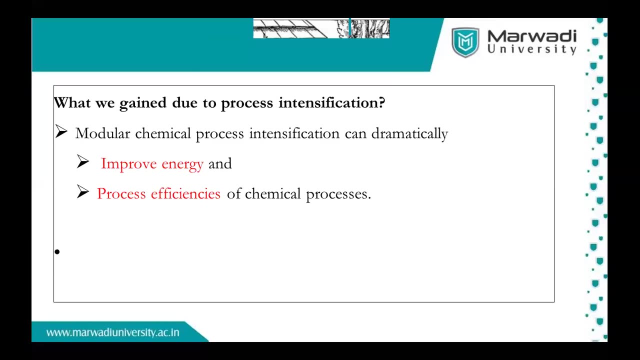 Is The Technology From 16th Century. So, Just To Go To The Next Part Which We Are Going To, This, So What We Have Gained. 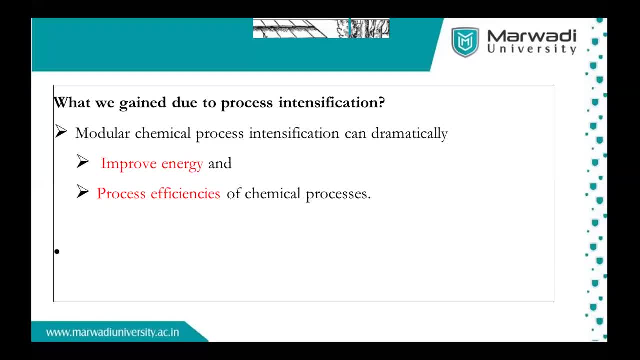 Due To The Process Intensification. Yes, These Are The Very Important Point Which We Have To Discuss. One Should How To Improve Its Energy To 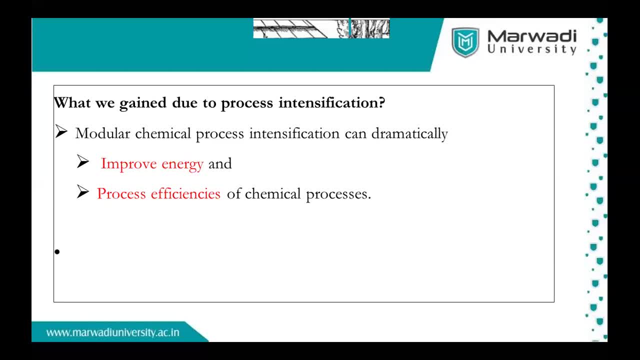 Convert That Raw Material Into Desired Marketable Product. So, As You Are Aware, It Can Be Done With The Help Of Different Kind Of Machineries. 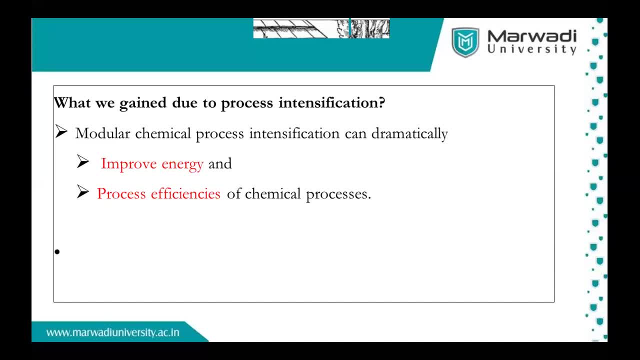 Different Kind Of Process, One Of The Definition. In One Of The Definition He Has Discussed About, There Will Be A Dramatic Change In The 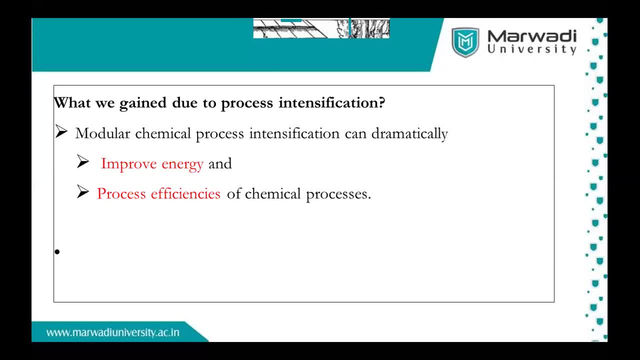 System Or Dramatic Change In The Process, Either It May Be Chemical Process Or Mechanical Process. It Is Going To Be Increased And That Is. 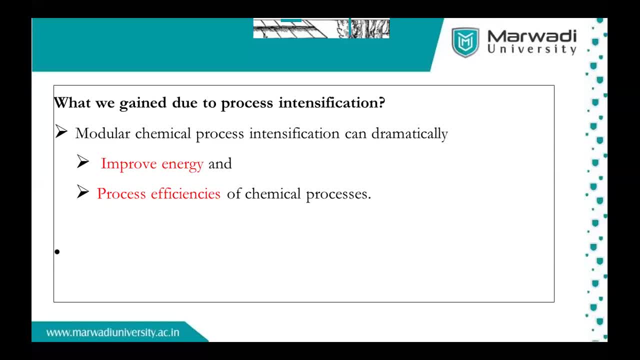 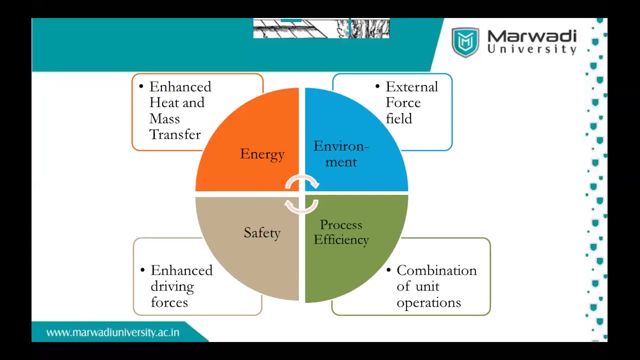 What The Our Aim Is Okay, So It Is One Of The Service Or Our 옵 S We Are Going To Use As A S. 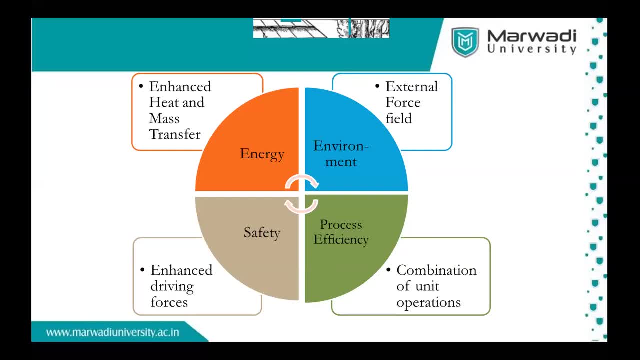 Management Or One Of Our Success In The System. So It Saves Time And Our that we have to maintain the safety features as well, as we should not hamper the features of environment. 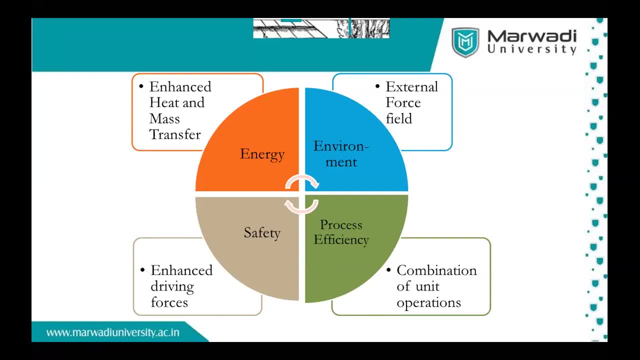 Okay, let's say this is a cycle. If you want minimum energy and maximum process efficiency, it must go through the different environmental parameters which we have to take care, and safety is also very, very important. So this is, let's say this is- the four quadrant of any process and that has to be taken care. 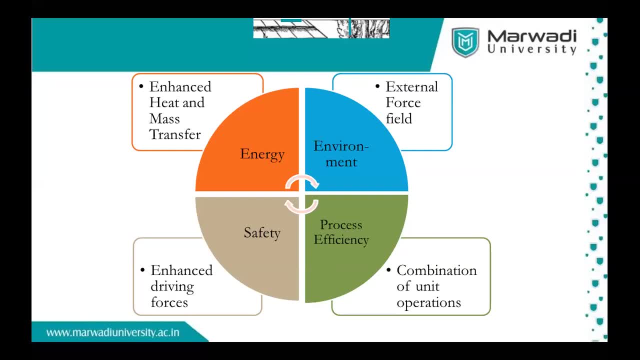 of when you will start your process right. So, as Dr Manish has already explained how to do the process intensification either, you can enhance the heat and mass transfer properties of any process, depending upon the nature of the system. right? Sometimes it is also said that when you are 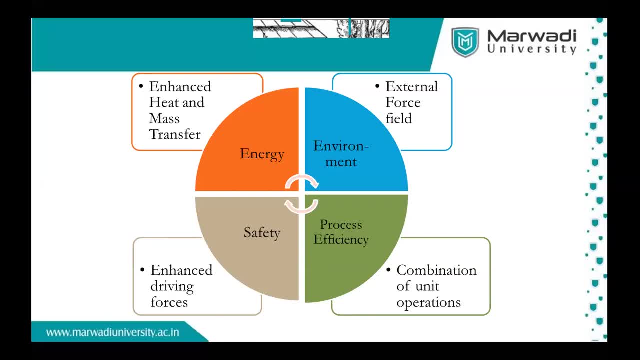 having less resident time. it varies again, it varies depending upon your requirement So you can have the enhancement properties in terms of heat mass momentum transfer right. Other than that, if you are aware about the driving forces, those are required. let's say, 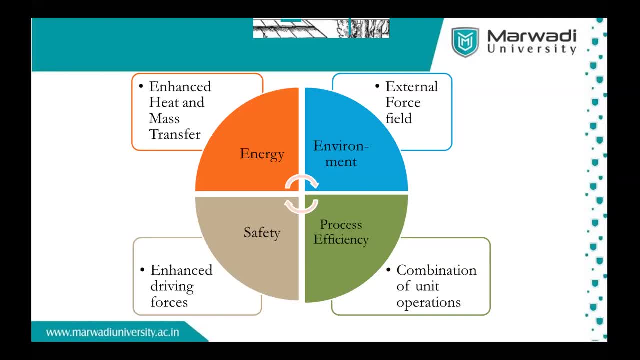 in mass transfer, it is concentration gradient. heat transfer, it is, let's say, heat transfer. okay, So there are different types of gradients. So enhanced driving force Also leads to reduce the resistance offered to the system. right Apart from this, we can combine the different units. 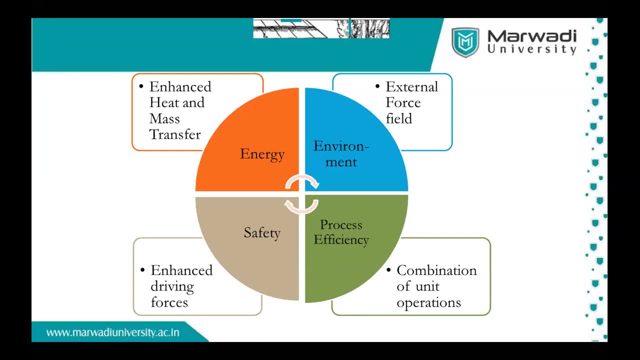 If you can remember the last image which I have shared with you from 16th century, you might have seen the different kinds of stir: tanks, stirs- those are connected to each other. You might have seen this, you might have heard about or you might have thought about what. 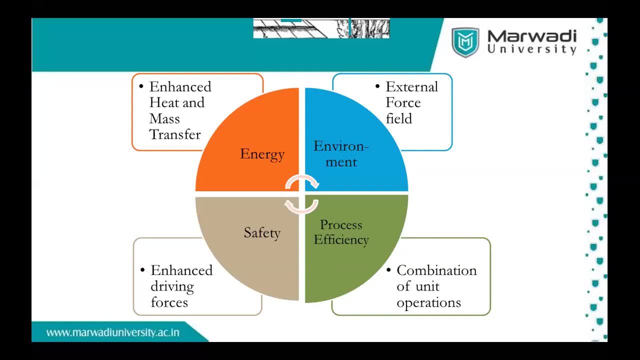 is a stir tank, If I can merge those- let's say reactors, pumps and so many other things along with those required, let's say parameters. so it is another parameter, let's say combination of unit operations, right And apart from this, new study has revealed that when we will go for external force field, 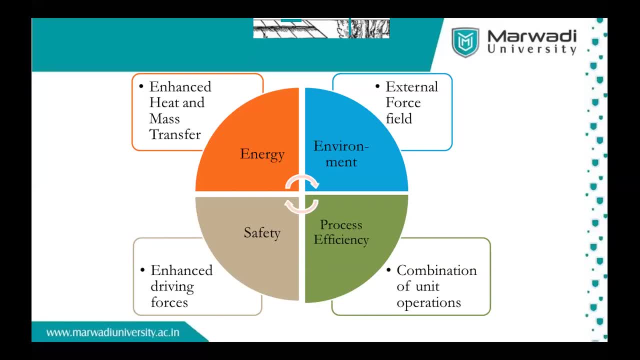 there are different kinds of external force field which may not be the case, Which may increase or decrease, let's say the rate of reaction, let's say very specific to the chemical reaction, and in many systems it required actually, either we may have to 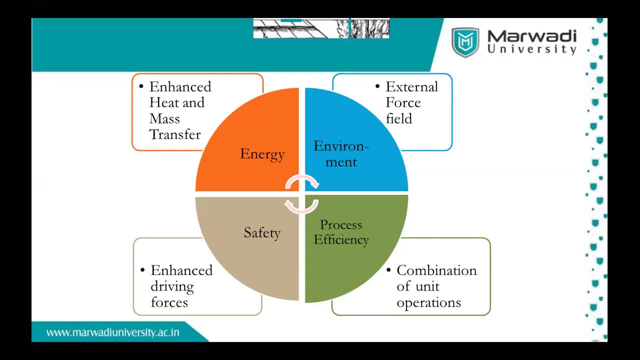 increase, or either we may have to decrease or we may have to keep constant some parameters throughout the your processing right. So external force field, let's say one of the technique is external influence, Let's say in terms of ultrasonic. okay. 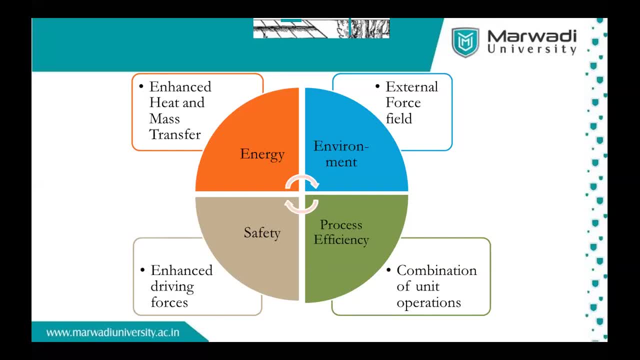 So this is one of the important thing which can be captured in nowadays in most of the industries, that is, implementation of external force field. So overall idea is, if we have to deal with process intensification, we have to deal with four important parameters. the first one is energy. second one is environmental aspect. 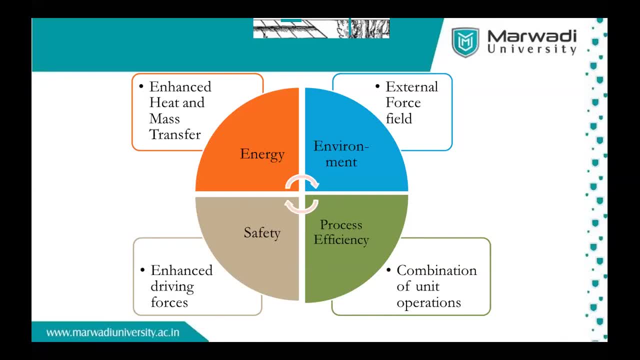 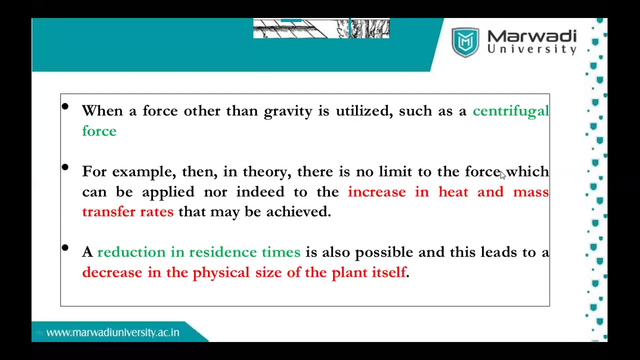 third one is process efficiency. And the fourth one is, at most, safety of, let's say, industry, as well as of environment and surrounding. Okay, So this is what the idea behind this slide is. Yeah, Yeah, Dr Manish, do you want to highlight this point? 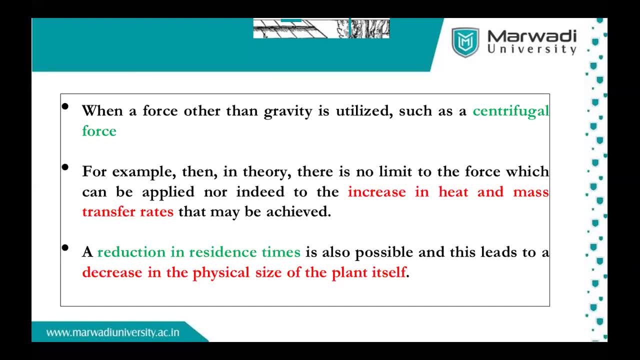 Yeah, Sir, Ritesh. sir, when we are talking about environment, external force field, now you can see that when force, other factors are involved. Okay, Okay, So there is no other gravity force other than gravity when we use centrifugal force, as, 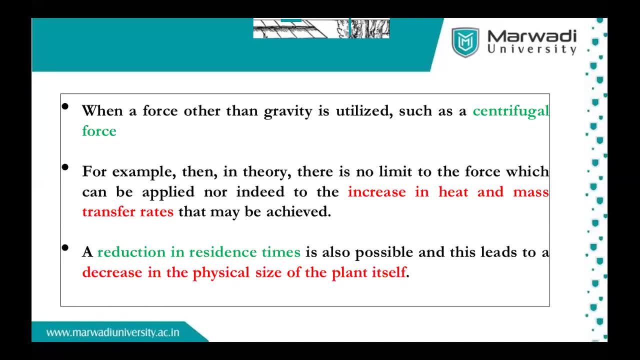 I told you the settling tank example rather than the gravity force. if we apply centrifugal force, then there is advantage of fast settling. The same way if we apply the centrifugal force in the what is called that separator- dust separator- and there you can see the settling of the heavy metal. 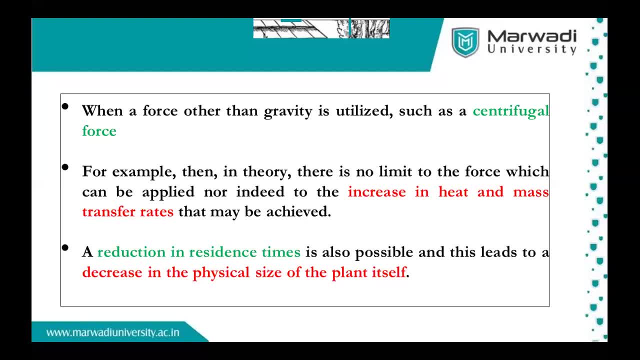 be, the rate of the settling will be faster than the gravity separation. so we can use this type of external forces to modify the process or to get the intensification. for example, if we apply the, but there is no limit about the force which you can apply. so in that way, as you do the changes, or if you apply 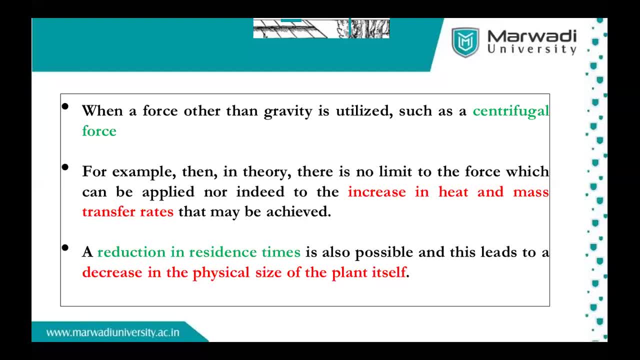 the centrifugal force or any other forces. the ultimate aim is to increase the heat and mass transfer rate. and once, if you are able to increase the heat and mass transfer rate, you are achieving the efficiency, you are achieving the this safety aspect, parallely and definitely you will get the advantage and you can reduce the size. 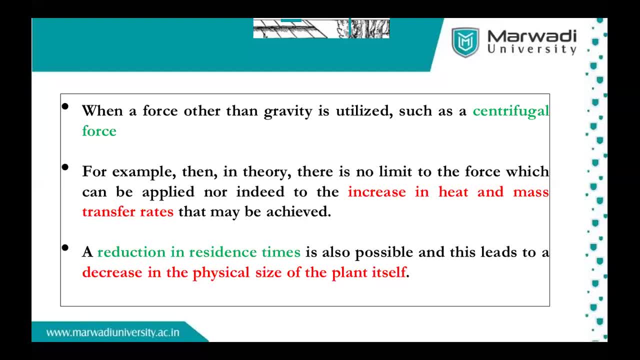 major. important is, once the rate of heat is increased or rate of mass transfer is increased, the same capacity which you are utilizing that unit, that unit you can reduce. you can reduce the size for the same capacity and automatically you are. the safety aspect will be improved, as well as the reduction in the residence time. this is very, very. 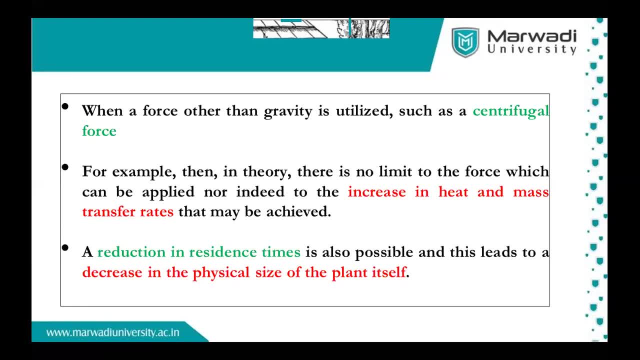 important. so then we, if you are able to increase the rate of heat transfer and mass transfer, definitely your how you are increasing the intensification. the same way, if fell able to reduce the residual, style means the rate of reaction. if you are able to increase definitely the residual stone, you can reduce otherwise definitely. there one 잠깐. 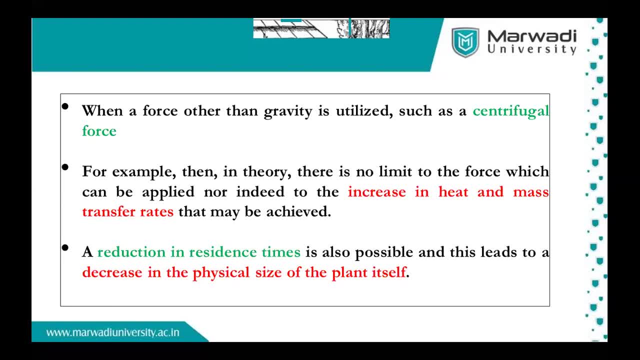 to direct both Progress. okay, so the resonance is very visible. so, for instance, the resistance, the difference is that i have included one favorable, that we". now we are all ready to proceed to the next project. ok, now, that is it. please feel free to click on the button below and like this video, or 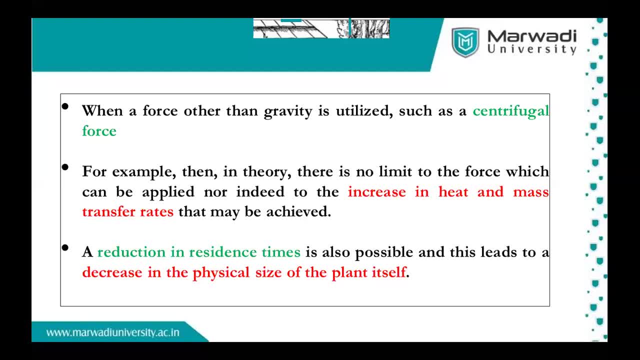 join with us at the end of the session. thank you so much for return to the online forum and in that way also it is possible to lead the reduce the physical size of plant itself. so major aim is to reduce the size of the equipment by applying 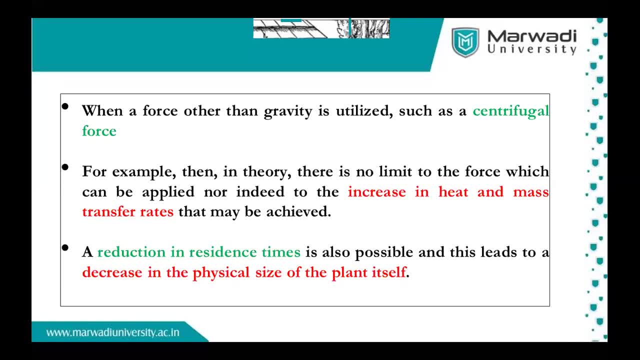 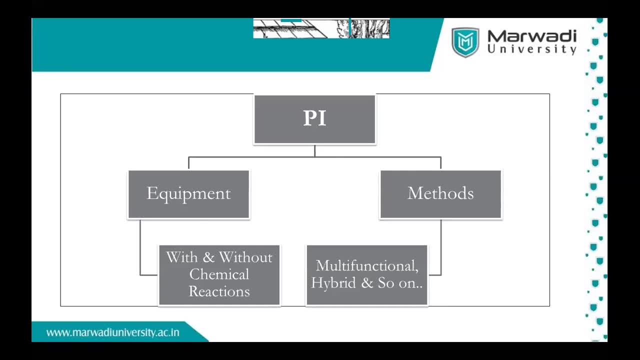 different techniques, as suggested by dr Manisha, that we have to believe the different kind of forces, as you suggested in terms of the example of settling tank, then the force which it is required in general, it is, let's say, gravity. gravity is the force which is required in general, it is, let's say, gravity, and 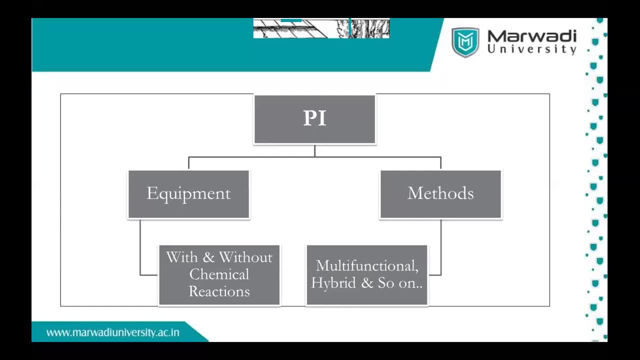 other than gravity, which kind of forces you can apply on the system and how to achieve the process parameters required. process parameters in terms of improved efficiency- that is discussed by dr Manish next. in general, you might have a question in your mind what exactly this P is. process intensification is right, so 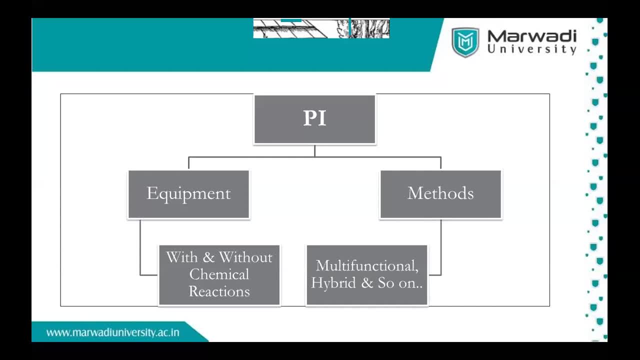 it is nothing, but it is a dramatic and drastic change in the process industry or in a process. so how it is to be done, or how that changes as has occurred in the system. so it depends on your methodology which you are going to acquire. so the first one: it may be based on the equipments, on and 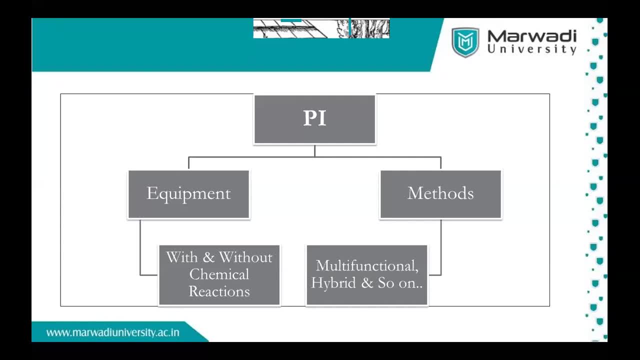 the second one, it is based on the which kind of methods you are using for your process. so let's say, equipments, which kind of equipments you may have. and if I will ask, if someone will ask you which kind of equipments you want as a chemical engineer, so definitely you guys. one of you will answer like that: yes, 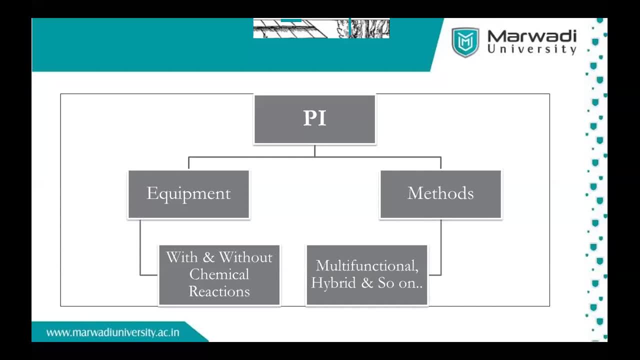 there will be some equipments where I can carry out chemical reactions. there are some reactions where I don't want to carry out my reactions, but at least there must be some change, as discussed by dr Manish, because as the processes or chemical reaction systems or chemical systems are divided into two parts, one is 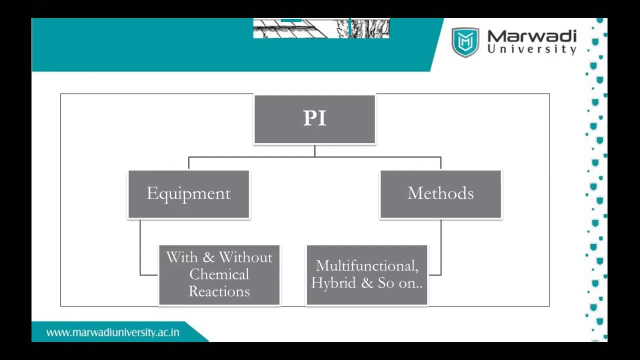 divided into, let's say, mechanical process and it's a physical process. somewhere you just want to crush it right. so sometimes there will be a chemical reaction, sometimes it won't be right. so equipments may be divided as without chemical reactions. which kind of methods you can use for PI? it may be. 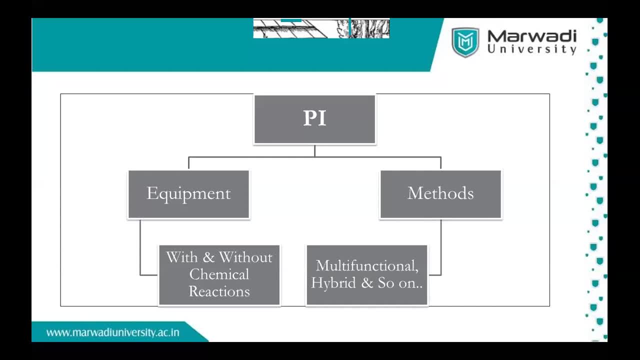 multifunctional right at the same time, if you are carrying out different kind of operations in a single unit, in a single reactor, right, so that may. we can say that is a multifunctional. one can say: I have to, I want to work on a hybrid. 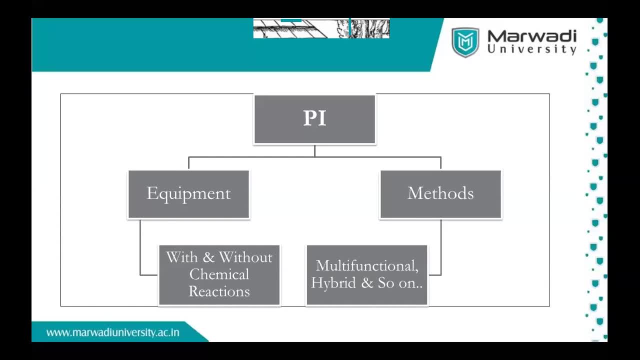 methodology. which are those? let's say, you are having conventional methods and if you are using some kind of membrane operations, right, so that I can say that is a hybrid operation, okay, and there are so many methods which are nowadays we are using in order to intensify our process. So, in general, process intensification, it broadly classified or broadly. 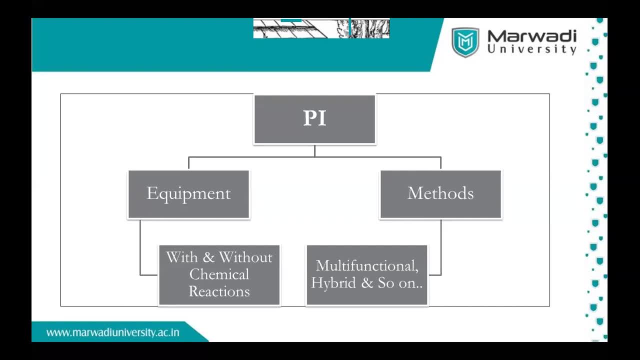 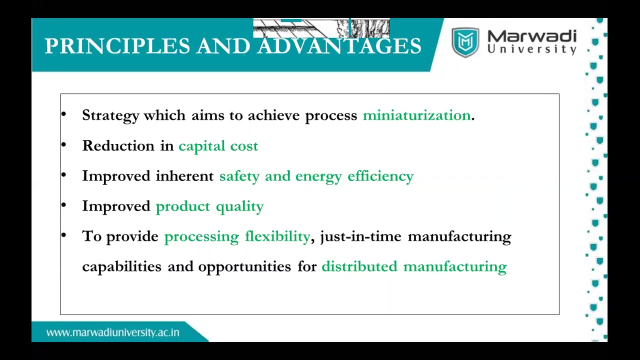 studied nowadays on the two aspects. that is based on equipment and methods. Next slide, sir, Just to move forward: Manish sir, next slide please Advantages. Yeah, yeah, yeah. So, as we have discussed about Manish sir, do you want to cover this part? 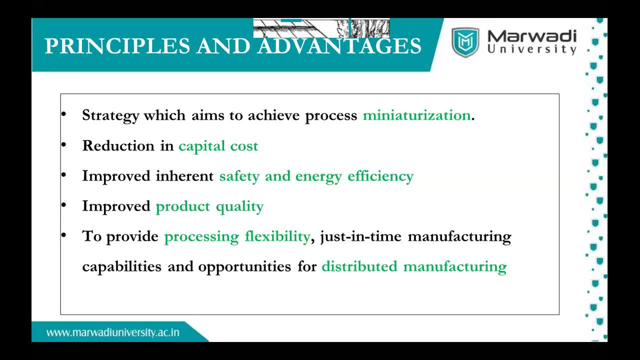 Hello, Okay, sir, Yes sir, Hello, Yes, sir, Please, please, So major, yes, sir. So we want to see the principles and advantages of the intensification. So we know the principles. So what are? the miniaturization is the major, important principle. 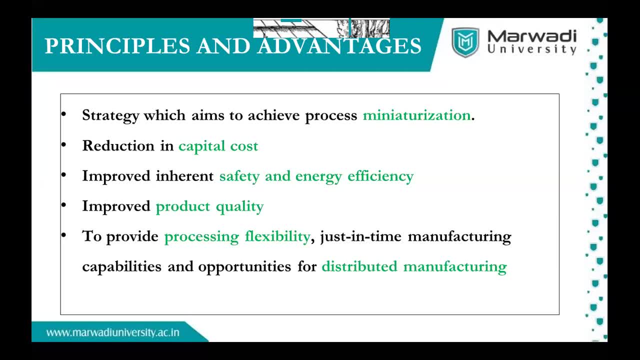 for this intensification And, as I told you, the reduce the size of the equipment as low as possible, so that the energy cost, as well as the cost of the equipment, will be reduced and the process cost related to energy mass transfer and other things automatically. it. 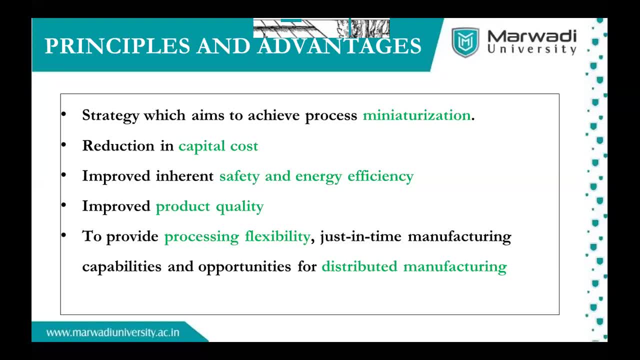 will be reduced by miniaturization And you can say it is the basic principle of the intensification. So automatically, with the help of miniaturization, you can reduce the capital cost. because capital cost if you see the total cost, if you, if you compare the total cost of the equipment, 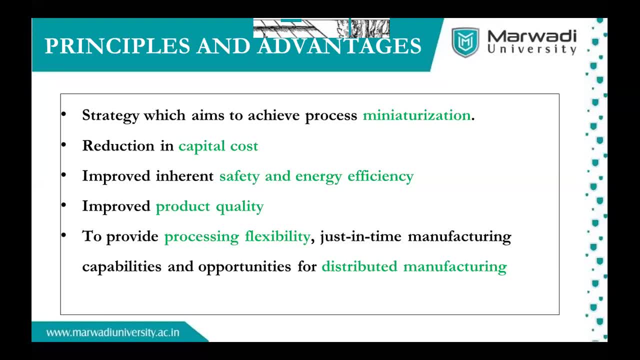 if you, if you calculate the cost of the industry, so major is the capital cost, because as the size of the unit is big, the cost of that unit will be more and more and it covers the capital cost. So you can reduce the capital cost in that way. Then automatically the safety. 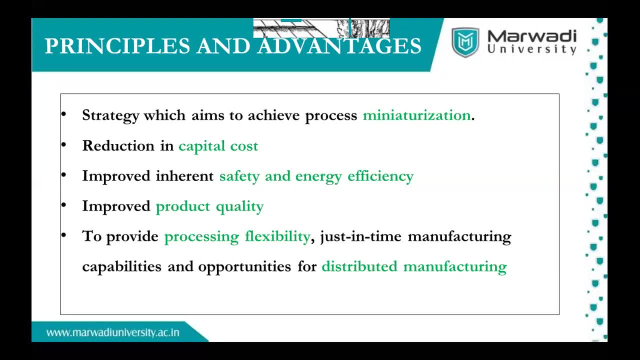 and energy efficiency. you do the handling of the small unit and the handling of the big unit. safety aspect it covers automatically. So it will cover the safety and automatically energy efficiency. Energy requirement will be less in the small unit, if you are able. 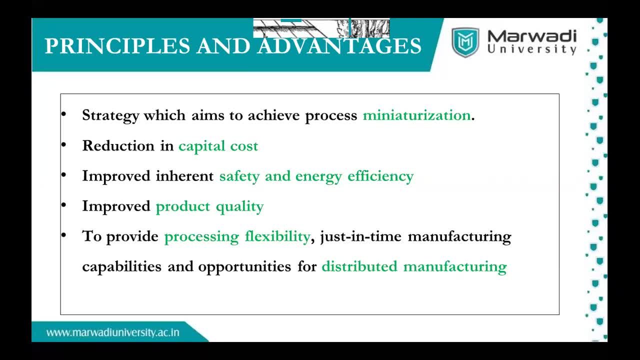 to maintain the same capacity in the small unit. Then you can focus on the product quality you can monitor very nicely in the small size as compared to the big size. So control, process control will be more. you can say it will be more controllable in the small capacity as compared to the big one. So automatically. 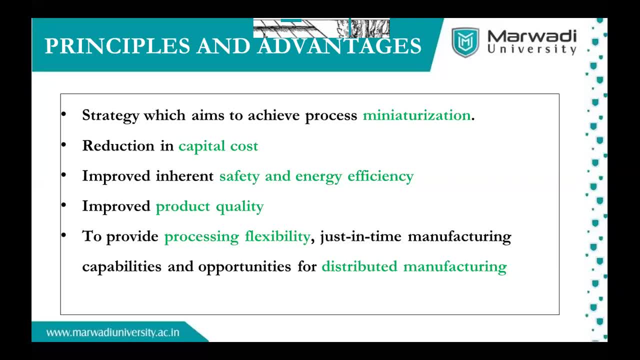 the product quality, it will be improved. Then next is process flexibility. Flexibility means what, Whenever most of the industry, there will be the change over, change over of the products. It is not the thing that the only one product can be produced in the one. 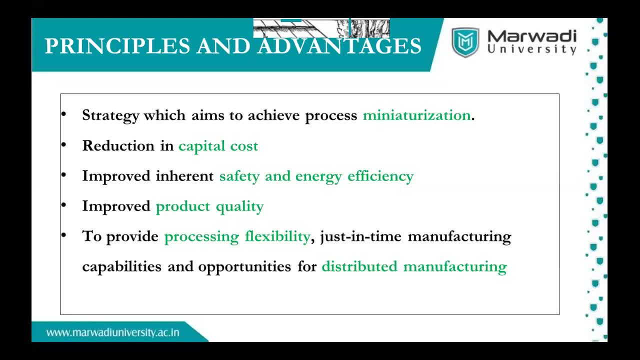 plant. There are different categories. You can say it is a derivatives, derivatives of the product, And whenever you are change over the products, you will have the flexibility. And when the size of the plant will be less or the size of the equipment will be smaller, 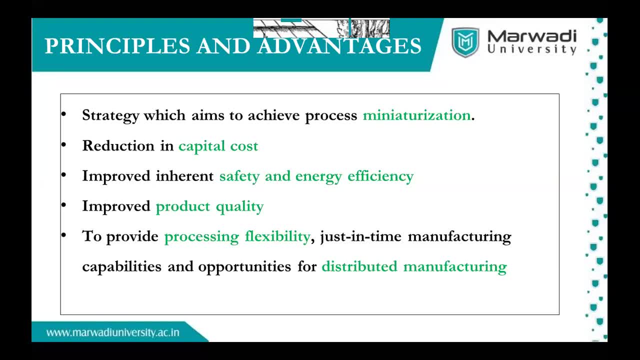 you will get the more flexibility in the process And just-in-time manufacturing and manufacturing time automatically- obviously it will be manageable or reduced- And capabilities and opportunity for the distributed manufacturing. What is mean by these capabilities and opportunity? You will have the more capability and you will have the more opportunity to increase. 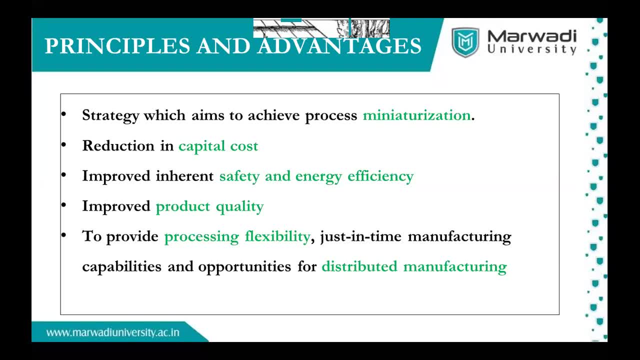 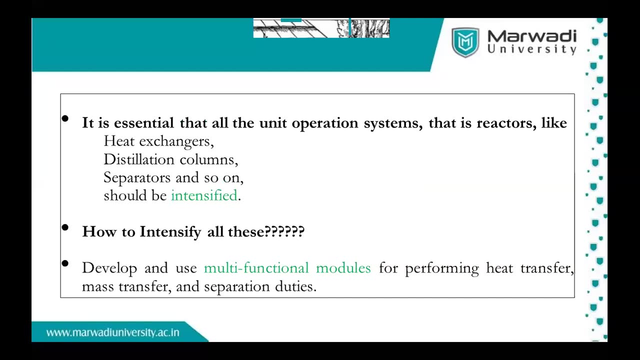 the derivative of the product. For example, if you have a small plant, you will have more flexibility in the distribution of the product. So these are the major advantages for this intensification process: Definitely, definitely, Definitely, as you have discussed in the last. 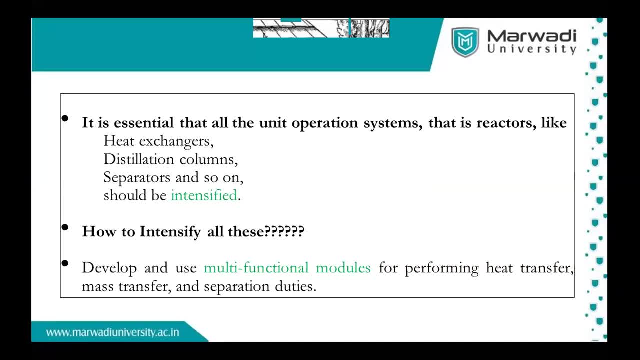 slide. there should be flexibility. One important point which has been highlighted by Dr Manish is flexibility of your process, along with your different kinds of process parameters. So let's say there are different kind of parameters, process parameters along with its components. So let's say we'll go with a very basic unit operation systems. 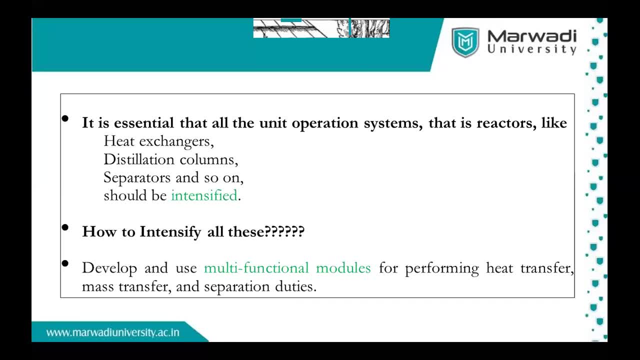 So we know we want different kind of reactors. those can be used for different processing units. So just for discussion. just for discussion, let's say we are having different kind of reactors like heat exchangers, distillation columns, separators, which already discussed. 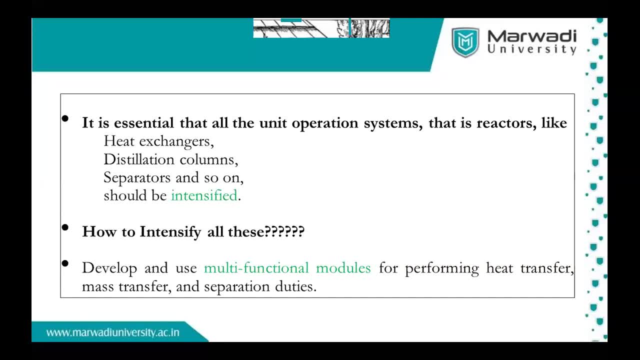 by Dr Manish. So if we will try to intensify those individual items in your process, your system is automatically intensified. So how to intensify all these things, As I had discussed earlier, that PI is done. It is divided into two sections. 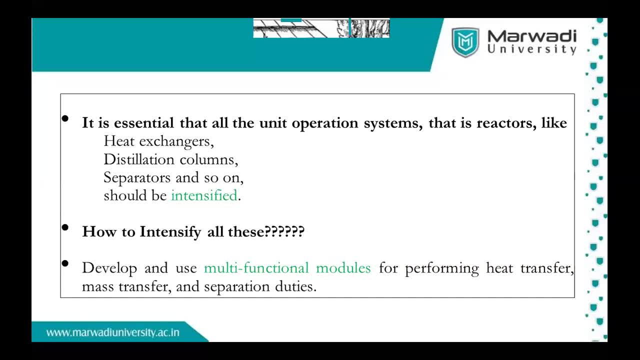 One, it is based on the methods and second, it is based on your- let's say- parameters, Okay, or let's say equipments. So very, very important is you must have multifunctional models, which are those modules. you can have a combined heat and mass transfer functionality, or you can have heat and separation duty on. 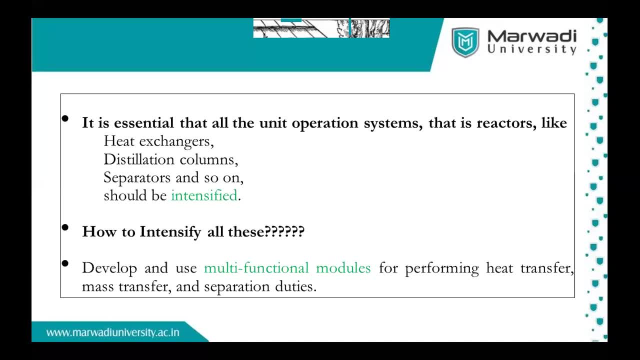 you can have heat mass and momentum, along with separation Right. Sometimes fluid may come into picture, Sometimes purification may come into picture. Sometime your cost may come into picture. So there are large variety of parameters, those we need to consider as a process engineer. 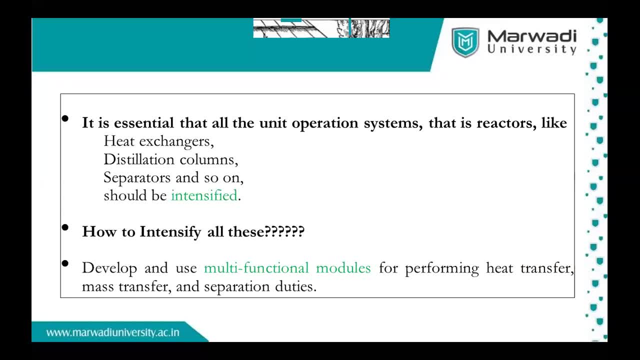 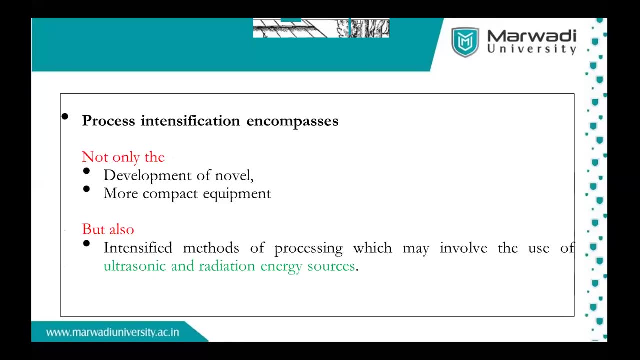 Okay, So these are the parameters which we have to discuss as essential and of, let's say, intensified. Okay, Next slide, sir. Okay, Next slide, sir, Yeah. But what exactly it is- You might be in a dilemma- that Dr Manish and Dr Ritesh- those are discussing about. 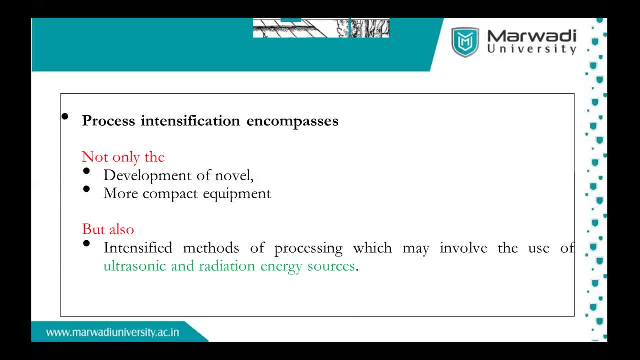 process intensification, process intensification and process intensification. But what exactly it is, What is its boundary, What are its limitations, What are its applications? Okay, So let us discuss in terms of let's say what it encompasses. Okay, 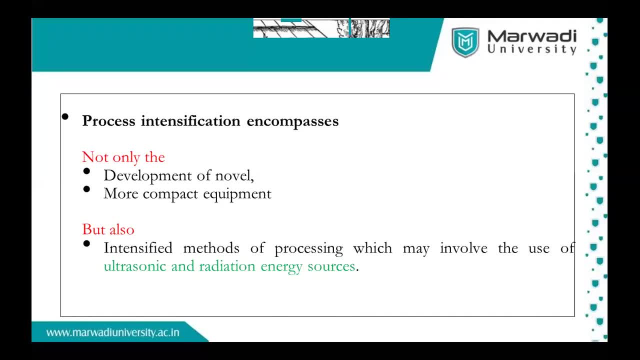 What is it? What it encompasses. So let's say, we, today, we want to discuss this in the form of not only and but also. So process intensification, it is not only the development of novel reactors, novel systems, Okay, Or more compact equipments. 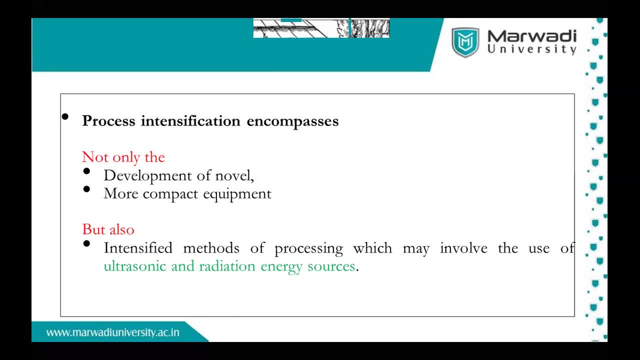 That is what Dr Manish has already discussed, that compactness, right or flexibility, but also it tries to. It tries to provide you intensified methods which can use the different variety of techniques that has not been used as a single unit. 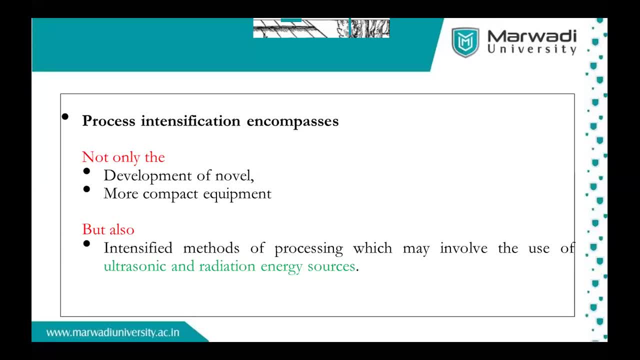 So one of them is, let's say, ultrasound technique. The second one is radiation. Okay, Just say the example of which Dr Manish has already emphasized on, let's say, for the reactors, In some reactions You may require heat. Okay. 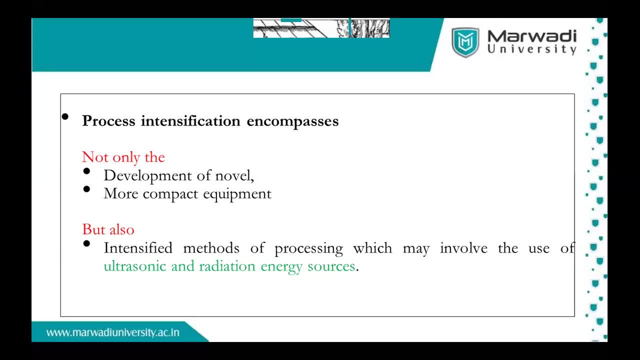 Heat Or somewhere you may not require the heat. Sometimes heat may be generated inside the system when the reaction is going on. Sometimes you want to give heat to the system from the or to the process from the outside. So these are the things. these are the things which we need to need to encompasses inside. 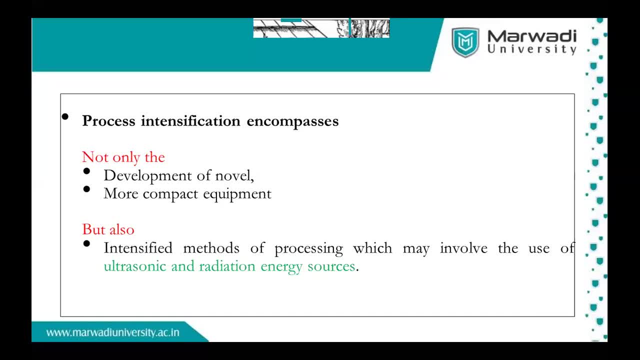 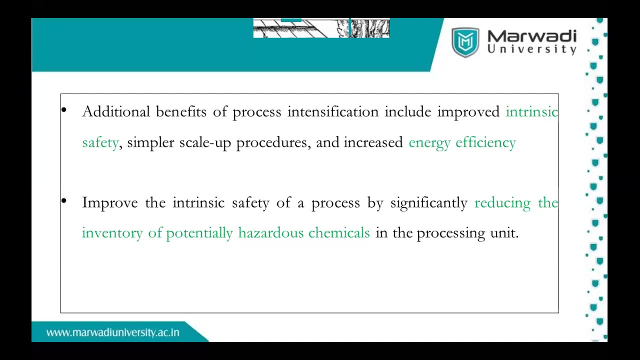 the system, Okay. So this is what all about. the process. intensification is Okay. Next slide, sir. So this is what we have to discuss about, that is, we want intrinsic safety and how it will increase the efficiency, or energy efficiency. So, though, we are discussing about the scale up of plants, along with the different kind. 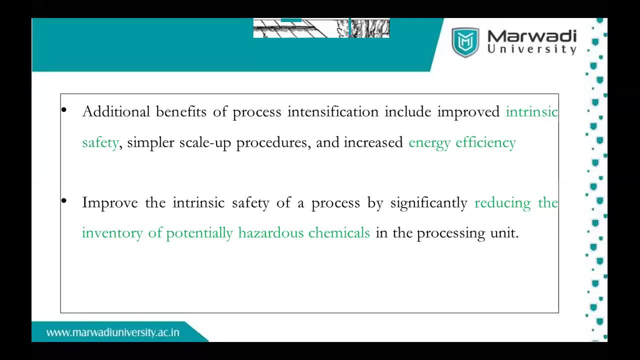 of reactors or unit operation and unit processes. it must be intensified along with the different different benefits, Like safety and energy efficiency, which we are emphasizing or which every inspecting body is emphasizing on nowadays, Right. So it is very, very important that we have to add those inventories in a such a way that 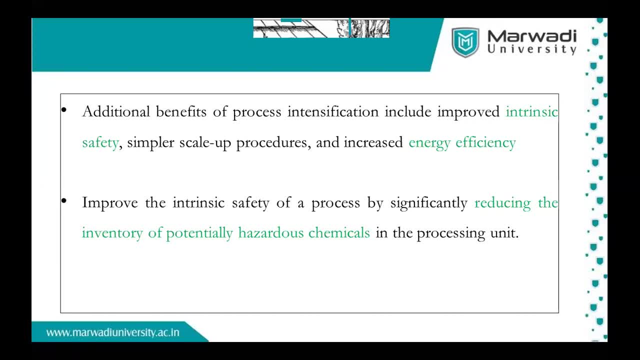 which will reduce the hazards, Right? So either it may be unit operation or unit process, Okay, Okay. So in terms of unit process, we have to deal with the parameters where we can reduce the hazards. Either it may be in terms of any kind of hazards which we can discuss in terms of SHC. 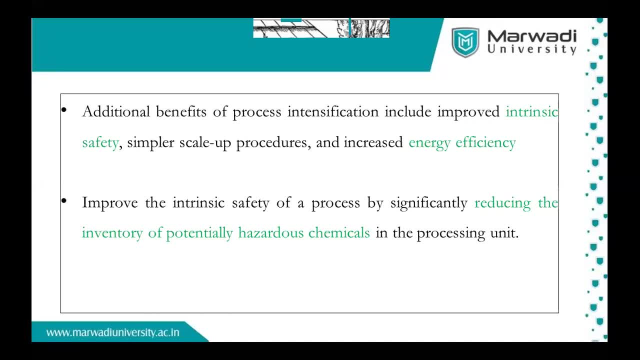 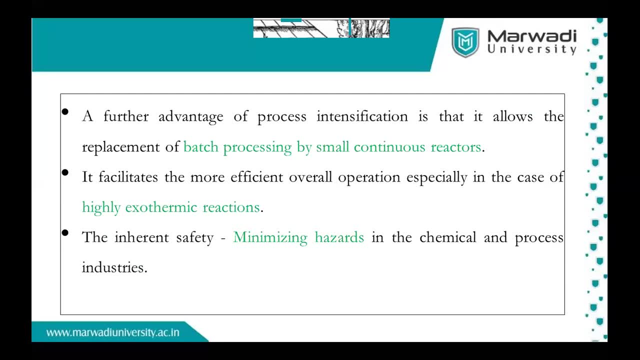 Right, Yeah, Next one, sir. Yeah, These are the advantages, as Dr Manish has started with the, let's say, a very simple example which we, as a beginner, can emphasize on. So what is the advantage? There are different processes, which has to be carried out in batch mode, or either it. 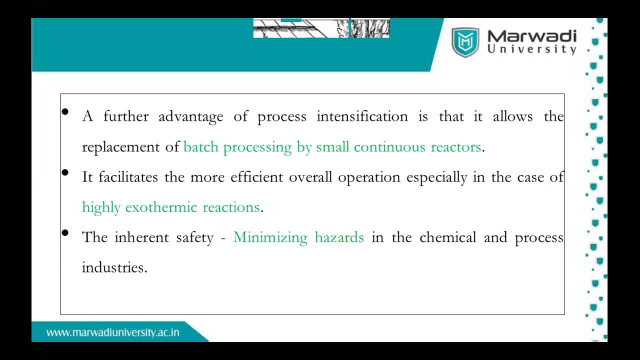 is in continuous mode. So can we alter the situation? Can we increase our production, Can we reduce our inflow, Can we decrease some kind of- let's say a day's every day, Right. Let's say intrinsic parameters, right. 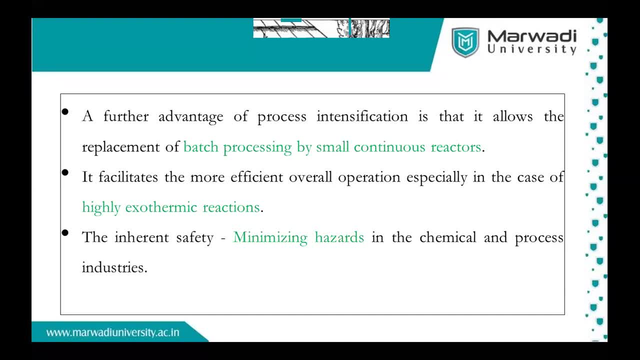 So this is what one of the parameter, the process engineer, may look after, that there may be inter conversion between the process parameters. So first one, let's say we can change, or we can switch to the batch, we can switch to the continuous process, right? 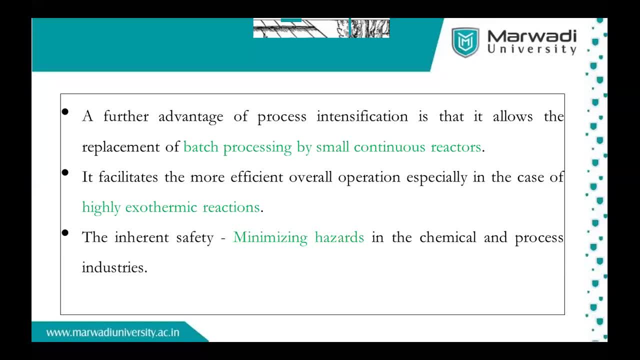 So what it can? it can facilitate, it may have more efficient system either way, And it minimizes the hazard. okay, so this is what we want to emphasize as a part of discussion in process intensification: that we have to increase the efficiency. 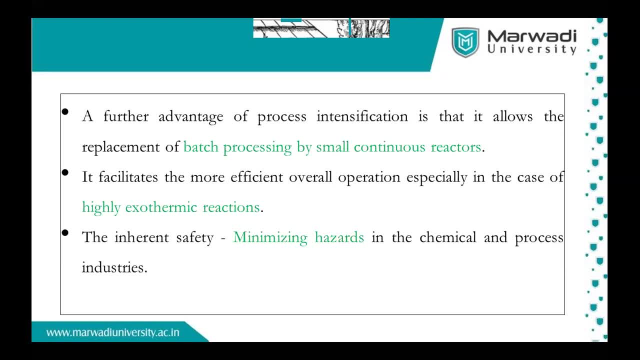 But at the same time, we have to reduce the hazard. it may be of any kind. Okay, Yeah, Next one, sir. So I would like to highlight this: you share some more information about this: how to convert the batch process into continuous reactor and how we benefit, how we get benefit with 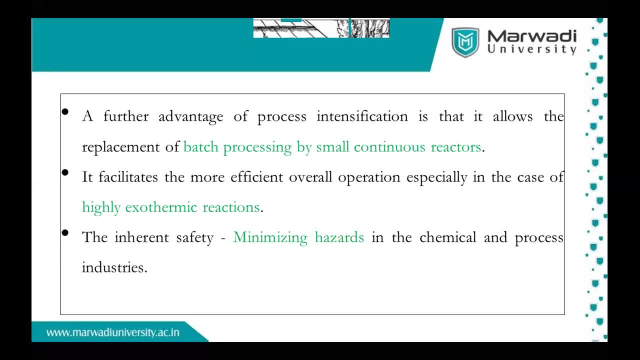 respect to the exothermic reaction as well as safety purpose safety aspect. So in my last when I was working in industry, we used to do epoxidation In batch. Okay, So definitely it was the highly exothermic reaction and that exact exothermic reaction. 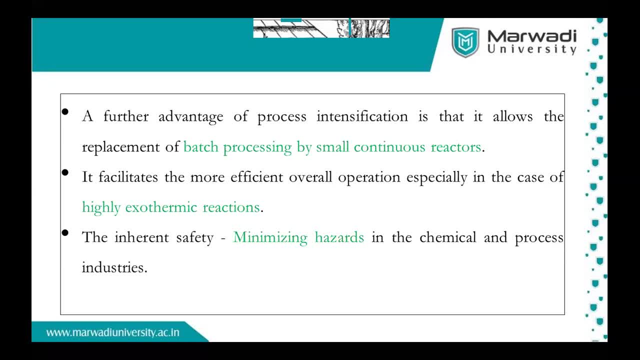 they want to convert into the continuous mode and we took the small packbed reactor And in that continuous packbed reactor when we succeed the conversion of batch to continuous, that exothermicity we we would complete that Okay control very easily because the small amount of reaction taking place continuously and 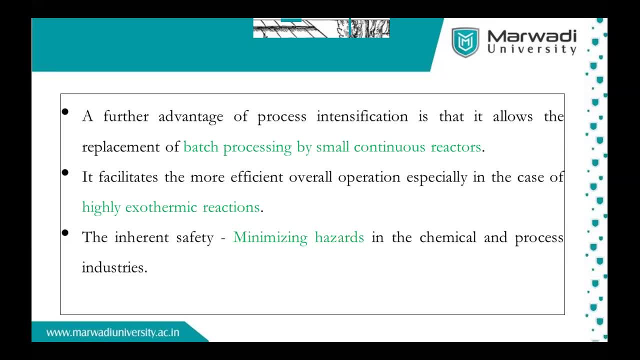 we are continuously controlling the exothermicity as well as it is the highly explosive reactions because they are using the peracetic acid and peracetic acid is more dangerous than the even hydrogen peroxide also. So we converted the reaction and we got the benefit of the rate of reaction. 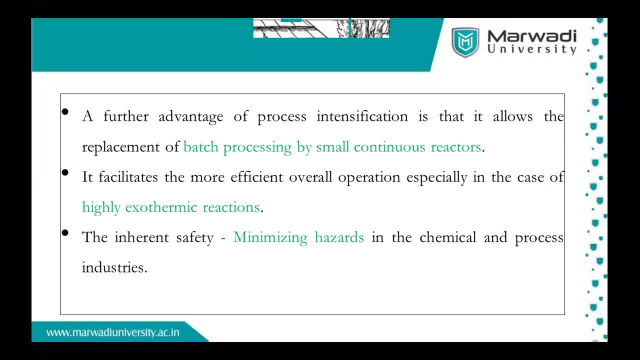 The unit size. instead of 10 kiloliter reactor we converted exactly into the only 10 liter in the continuous form and, moreover, the labor also we have saved, how taking that reactions and taking into the distillation and again purifier instead of that continuously, because 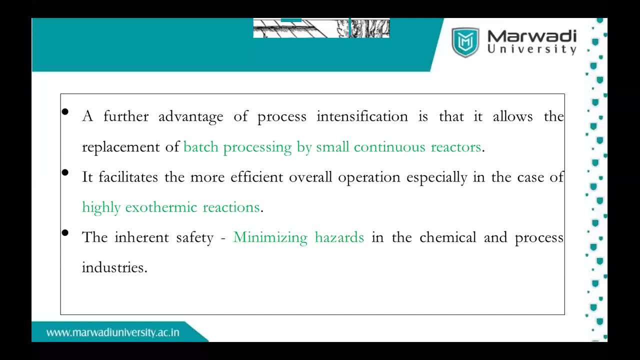 it is the. So as soon as the reaction finish, we send into the small distillation in it and distillation online taking place and we got the three benefit: one is the efficiency, another is the safety and third is the controlling of exothermicity, which is more related to the hazard also. 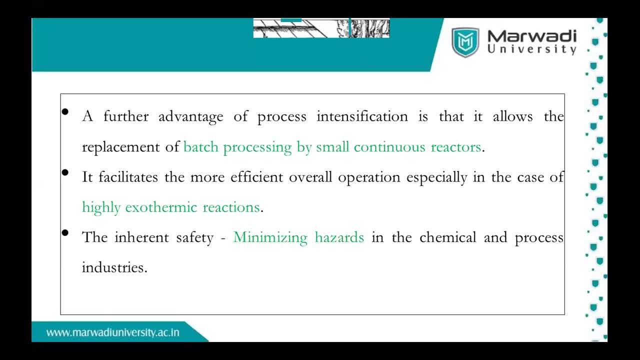 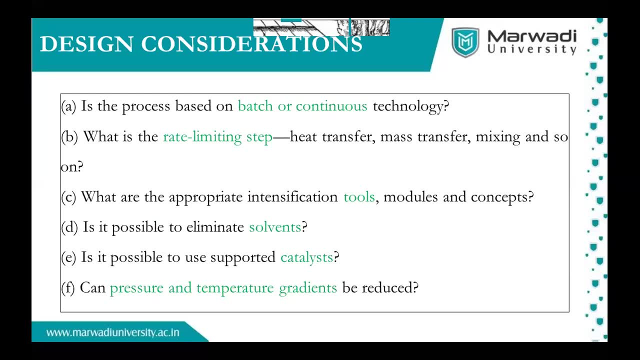 So this is the best example of the intensification process: the conversion of batch into the continuous. Yeah, and that is what the Manish sir discussing about, how they have converted the batch process into continuous right. so let's say, to be a technical graduate, we have to deal with the 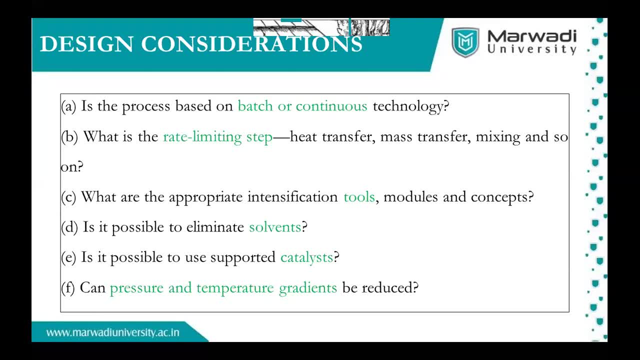 different kind of design parameters or design considerations. okay, so let us start with the very important discussion: What are the design considerations? right, because as an engineering graduate, we have to look for different aspects, so desire, let's say. this will be a bucket list for any engineer. 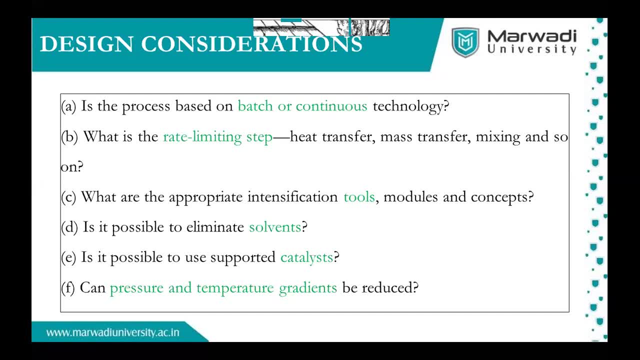 that if you want to do a PI for your process, what should I do? initially, I will go to the literature, I will go to the various examples said by the other industries and I will try to put my perception about that. So Yeah, As we discussed earlier, either whether is the process based on batch or continuous right. 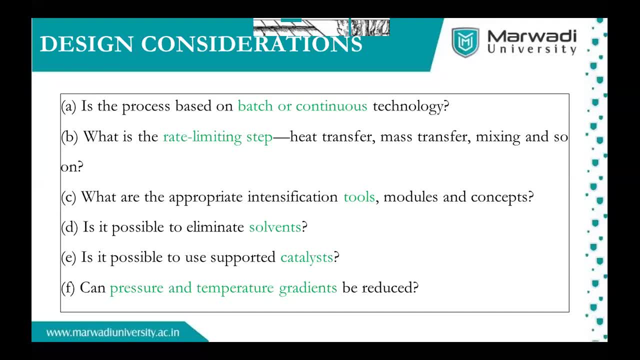 so that the next, and very important, as a chemical engineer, whether do this process is having any rate limiting step? it may be in terms of heat transfer, mass transfer, mixing and so on, depending upon your process. right then, if you are aware about key I have, let's say, 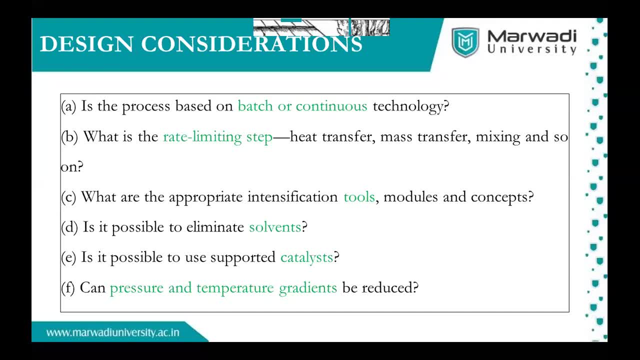 n number of parameters, N number of equipments which I have intensified, but which kind of appropriate intensification tools I can use so I can create my own modules? what will be the concepts I need to implement? okay, so in some of the processes, as Dr Manish has already said, the safety is of utmost importance. 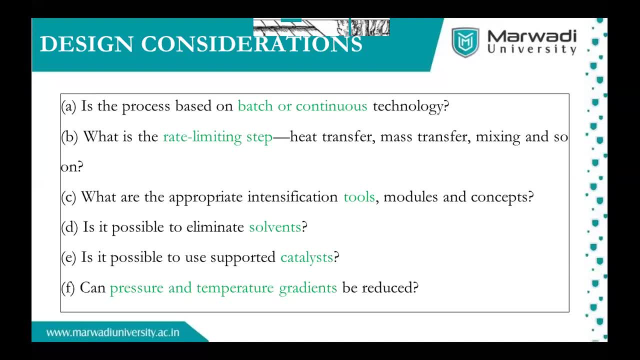 so can I reduce any kind of chemicals? Let's say you can eliminate any kind of chemicals. Let's say you can eliminate any kind of chemicals. Let's say you can eliminate any kind of chemicals. I will explain the solvents. okay, if we are using catalyst, how it is supported inside. 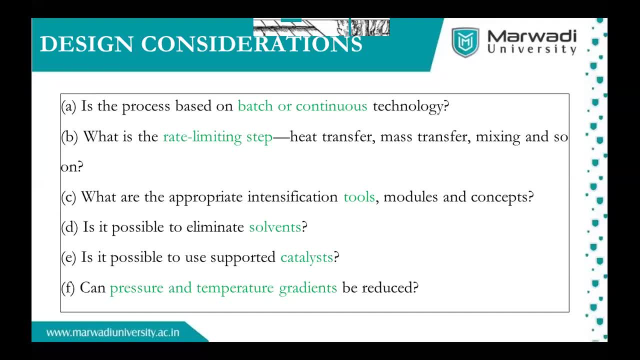 the system or how it is supported outside the system, how it to be a, let's say, packed inside the bed. So these are the different parameters related to the CRE. Next, and very important, let's say, if we have to discuss in terms of thermodynamics, can? 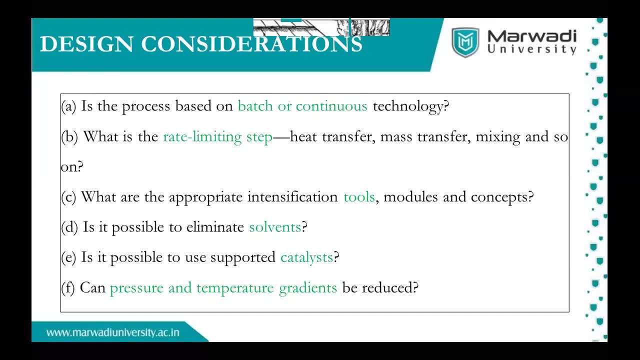 we reduce the pressure and temperature gradient, As DrManish already discussed. Okay, about the process intensification processes, One of the literature. it is mentioned that our system has intensified in terms of its space process parameters optimization up to 100 fold Right, So this is all depends upon this, whether it is batch or continuous. 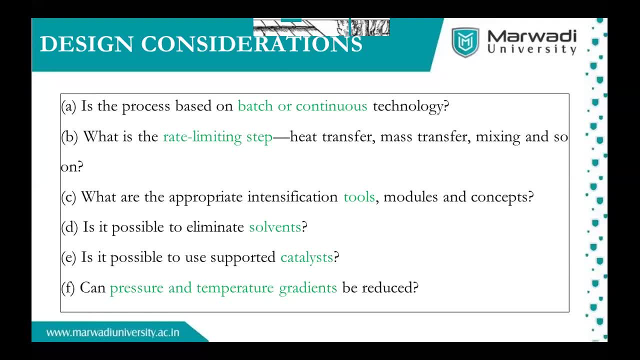 process. you are having different kinds of tools, modules. you can either eliminate one of the reactant. you may have different kinds of catalysts- Okay, And based on thermodynamics- whether you can reduce or control the pressure and temperature gradient- Okay, There are. 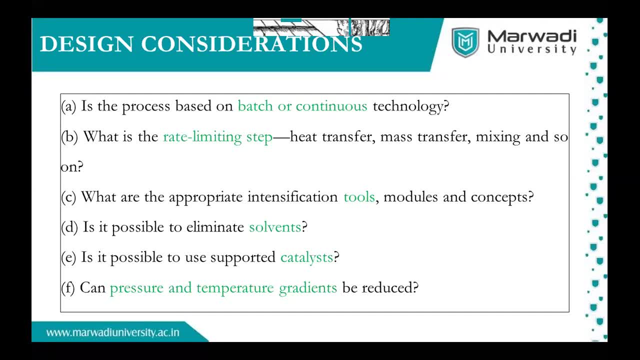 different techniques. but as this is basic, we are not going in detail. Yes, sir, Do you want to add something, Sir, I want to highlight. Thank you, sir. Again, I remember that solvent eliminates solvent point. So in batch reactor they used to take toluene. 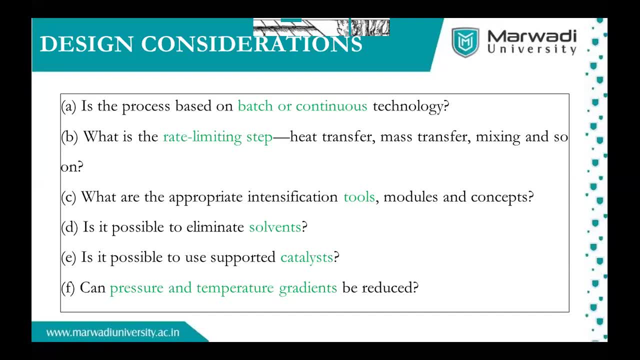 And the catalyst was sodium carbonate for the epoxidation reaction. But when we designed this pack bed, so we took the Lewis acid as the catalyst. it gives the very efficient rate of reaction And we removed the toluene. Okay, so the it is helpful to reduce the energy. 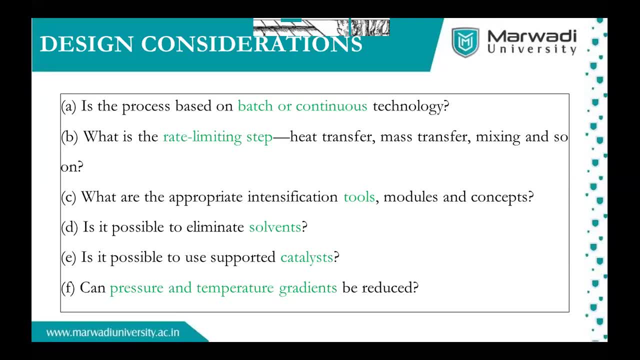 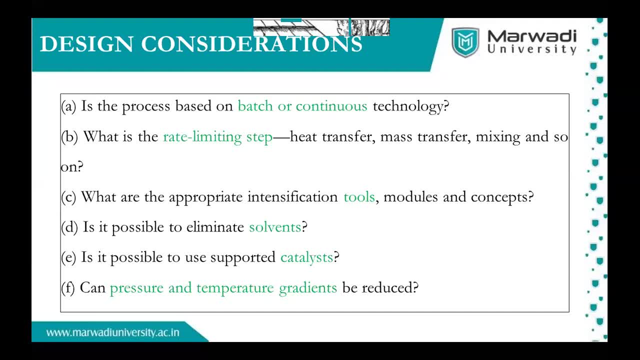 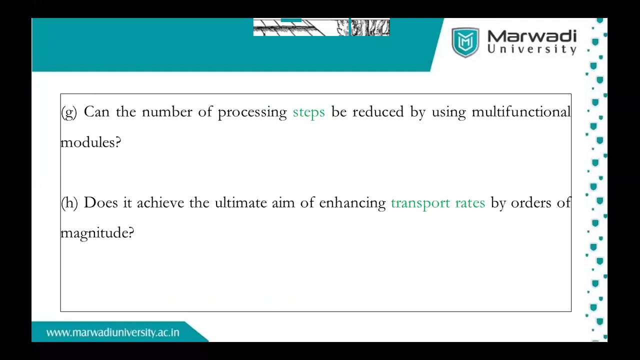 Yes, Yes, Yes, Yes, yes. That was a very important part When we took the design intensification. we can remove the solvent. Okay, Okay, Okay, thank you all. to remove the solvent, if possible. apart from that, let's say how many number. 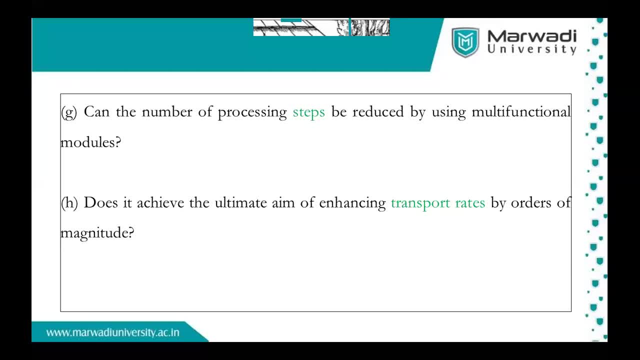 of stages we have, we can have. so let's say sometimes what happens, though you will work on different criteria to have a multifunctional modules. there may be some loopholes, right. so how to rectify those or how to identify those, how to troubleshoot those right and 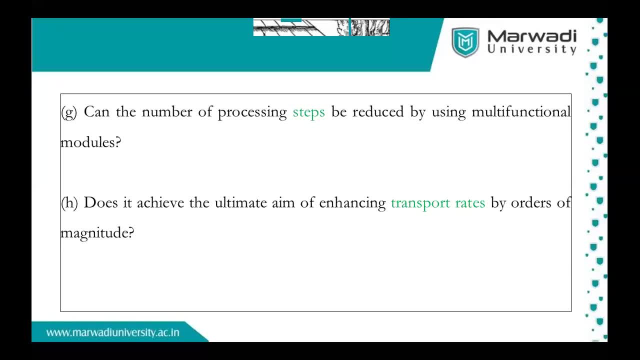 let's say how to enhance my transport rate as a chemical engineer. we have to discuss about heat, mass, momentum transfer. so how to deal with all these parameters and what are its, let's say, correlation with other parameters. so let's say, if someone is saying that pi 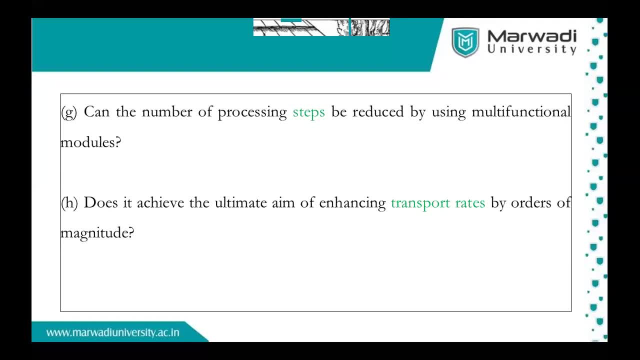 is necessary as my personal view. yes, pi is very, very necessary, but it can be implemented only and only after a detailed study, detailed plan and detailed blueprint, otherwise your system may fail okay. so these are the all design parameters which one can decide, as once again, i want to highlight, as we are discussing, 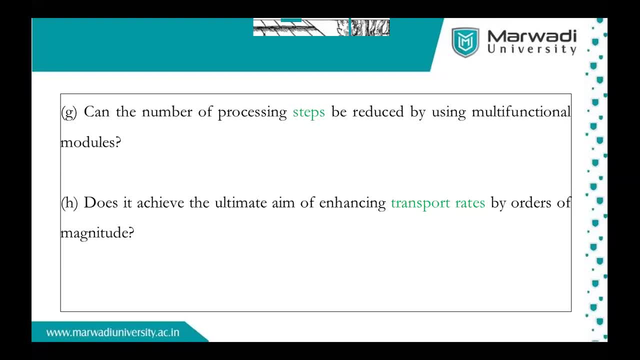 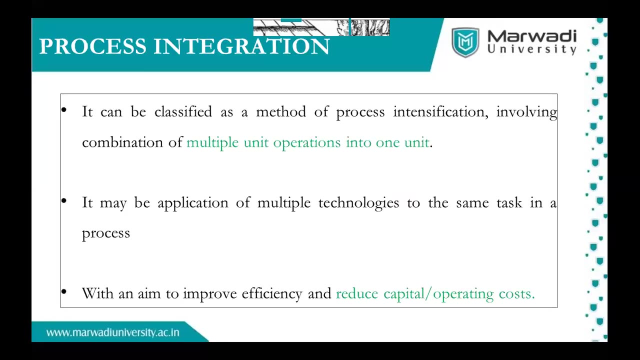 very basic things. these six to seven design parameters may change, may vary as far as the different processes as concerned. okay, yeah, next slide, sir. yeah, this is very important how to do the process integration. okay, so i would request manish sir, because, as he is having expertise in the process integration and he has worked, 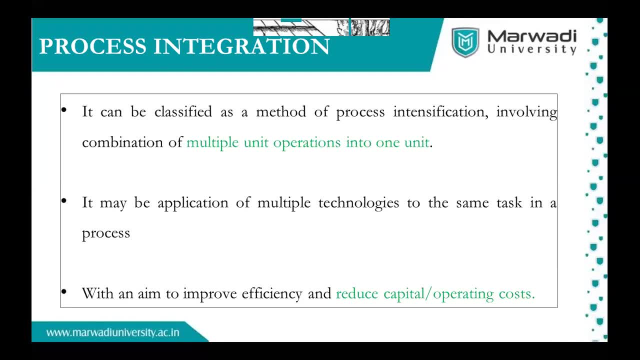 in different industries where he, under his leadership only, there are some parameters he has changed. okay, so he is going to go through the process integration, process integration. okay, so he is going to go through the process integration, process integration, process integration. So as an expert, he can highlight this. but I would like to request to you, sir, just 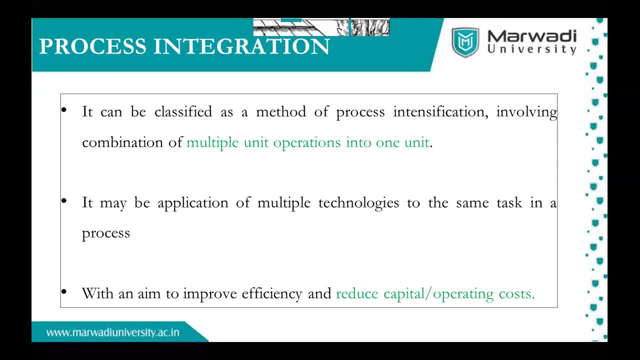 try to focus on only a few points as we are short of time. Thank you, sir. I would like to tell, especially in the unit reduction, individual unit reduction, and then we connect those units and when we make one process, so that process, whole process. 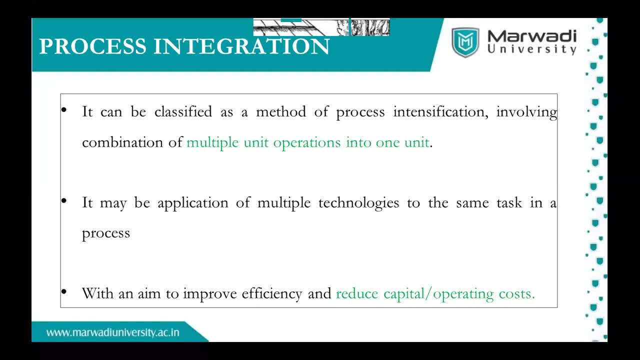 is called the integration, But basic is the intensification. So, and another point of integration is: we have to recycle, don't waste anything. For example, if you are using catalyst, you have to recycle catalyst in such a way that it will be utilized. 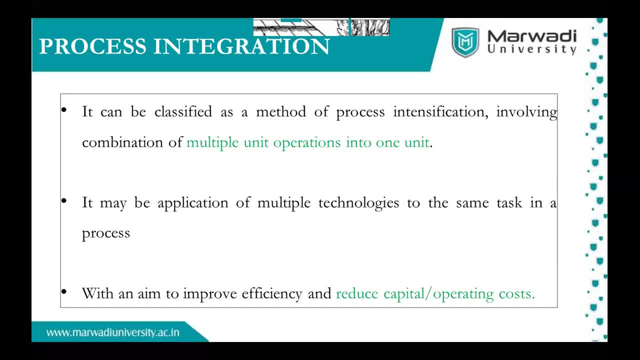 For example- I want to do short- In the paper industry they are using the sodium hydroxide and if you are not able to recycle that sodium hydroxide 20% solution for the cooking, it will be waste You cannot throw. environment will affect. 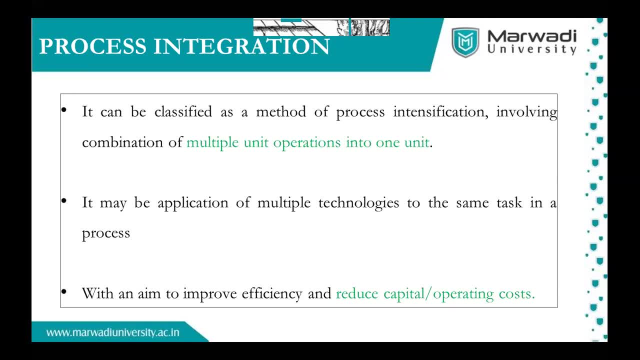 Safety problem will be there. environment problem will be there. So better to make another process so that it will be recycled, And while recycled you will get a lot of energy. That energy you can use for the making of the electricity As well. 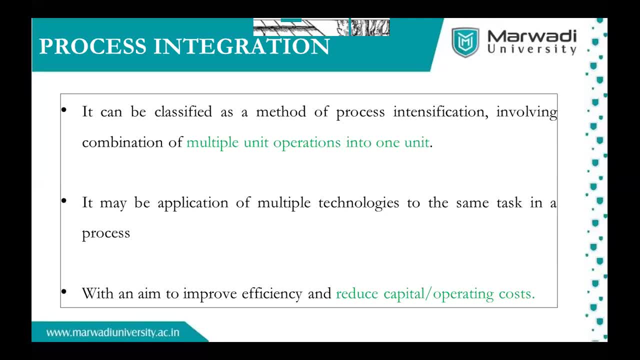 So 50% of the electricity you can make in the paper industry with the help of these two things. They say killing two birds with one arrow. So there are two benefits. you will get the two things. one is the recycle and another. 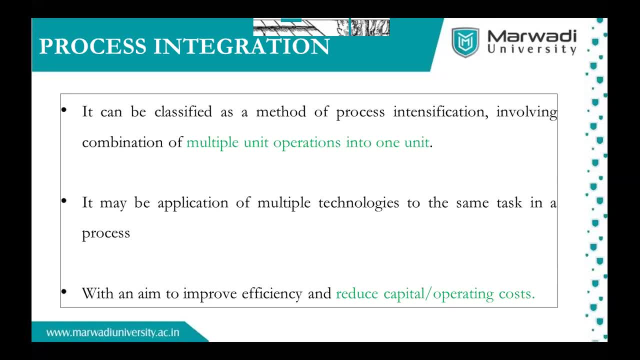 is the energy efficiency You will get the energy back, So this is called the integration process. It may be applicable to multiple technology as well as the individual also, And in that way you can improve the efficiency to reduce the capital cost as well as operating. 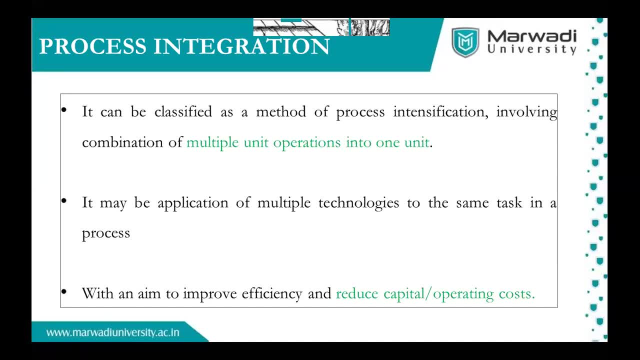 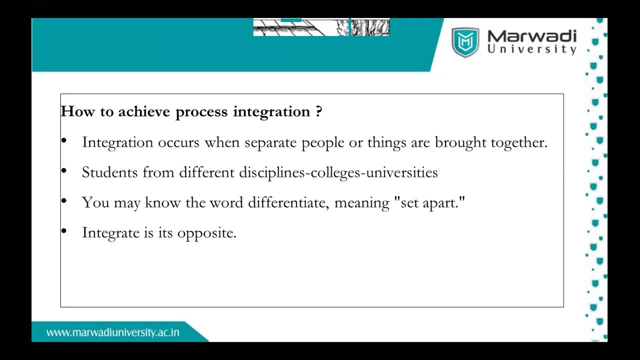 cost also. So integration is the next stage of the intensification. So how to achieve process integration? So you can achieve the process integration with Delphi. When separate people or things are brought together, When you bring the all small unit in the one unit, try to compact. 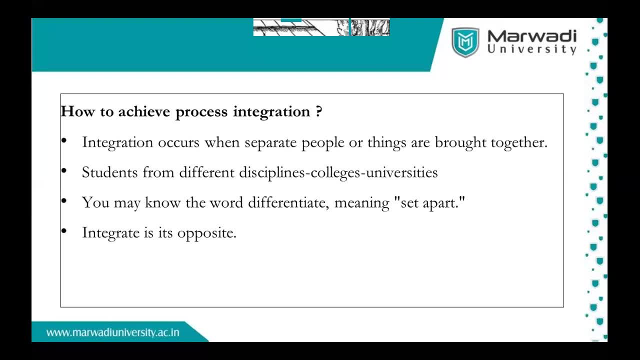 If you have 10 units, try to reduce into eight or try to reduce into five, So you can say it will be integration and it is exactly. you can reduce the size, also, whole process size, with the help of integration and it will give the lot of benefits. 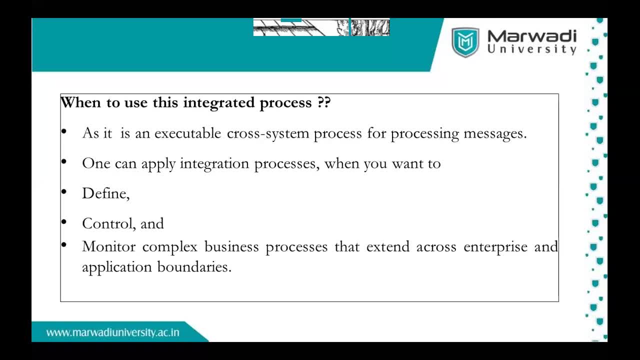 So when you use this integration process, you have to apply a lot of controls to get to do the integration and you have to execute cross system process sequence What can be done in sequence so that the process can be reduced. You have to monitor the. 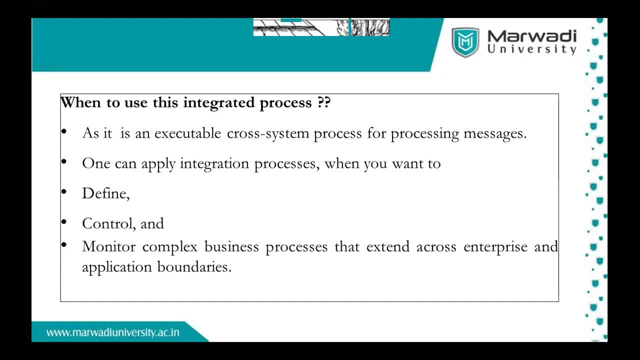 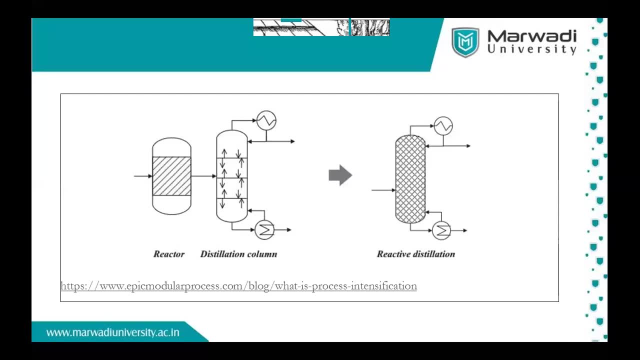 That process in such a way that you can reduce the size With a lesser. And this is the best example of nowadays distillation column. This is the research is going on how to convert into the reactive distillation. So the combination of the reactions and distillation all together in a one place. 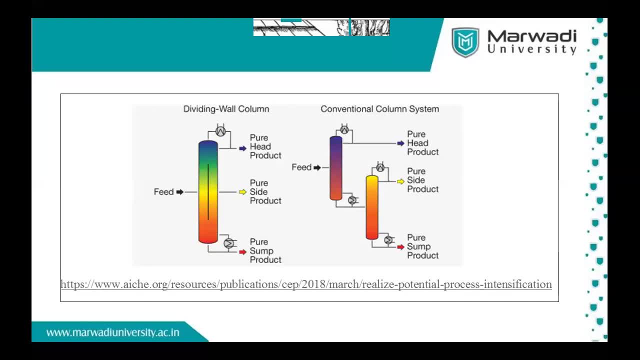 With this, sir. Definitely This is one of the best example, which already we have cited, where reaction and distillation is combined into one section So we can- it can- give a reactive distillation, Okay, actually a distillation itself. It is a big. 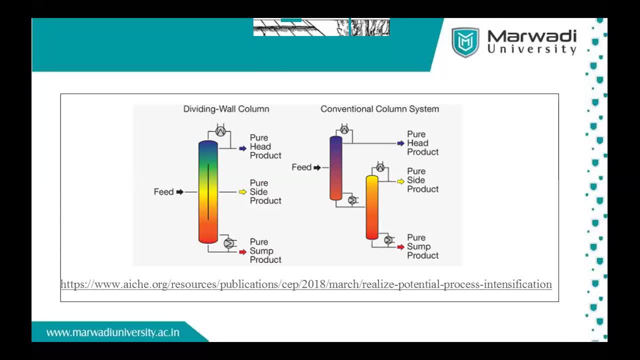 Let's say, industrial reactor, where we can have a different kind of reaction mechanism, and if we can combine that as a hybrid, As a process intensifier method, Yes, we will be benefited. and, as sir suggested, a lot of research is going on and already. 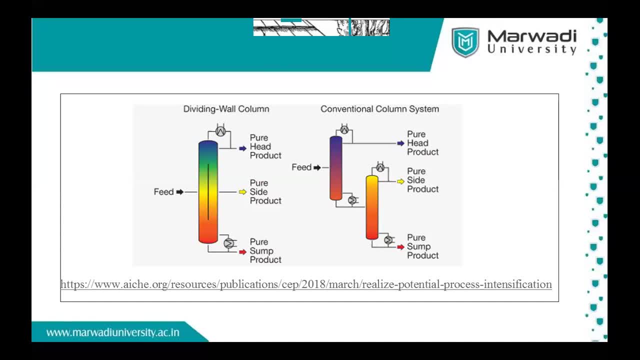 many of the industries has installed a different reactive distillation. apart from reactive distillation, There is one more part, Let's say for a dividing wall column, which is one of the PI Equipment which is Published by AIC HE and if you are able to see on the right side, that is conventional. 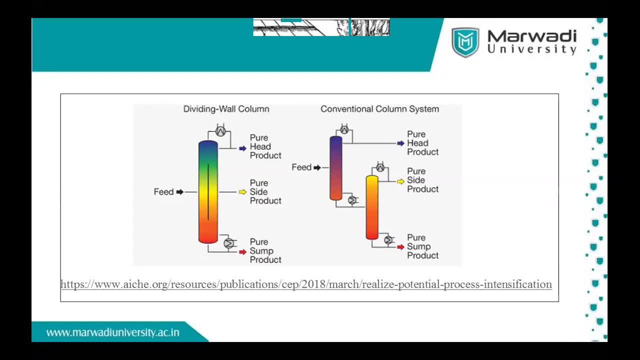 column system where a combination of two reactors then heat exchangers, then you are getting from somewhere, you are getting the product. either it may be pure, It may be impure, It depends. So what you want. you want more energy resources, you want more space, you want more collecting. 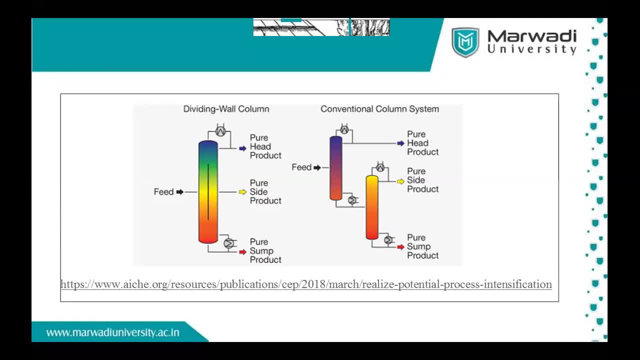 hands. you want actual feed And its location. if you are aware about the design consideration of distillation, you can visualize and analyze the situation to work on a distillation. But if someone come with combining of these two, these two columns, then what? there will be a dramatic change in a process. so one can get. 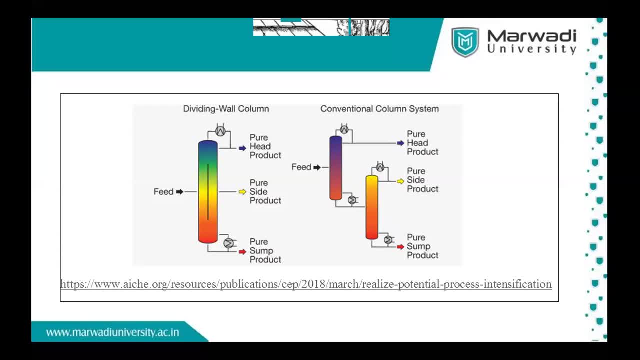 Increased. purity, efficiency will increase, energy will be reduced, Right Space will be reduced. Okay, So there are different parameters, which already discussed in the literature. as far as dividing wall column is concerned, Yeah, next one, sir. So as far as concerned with the system integration, 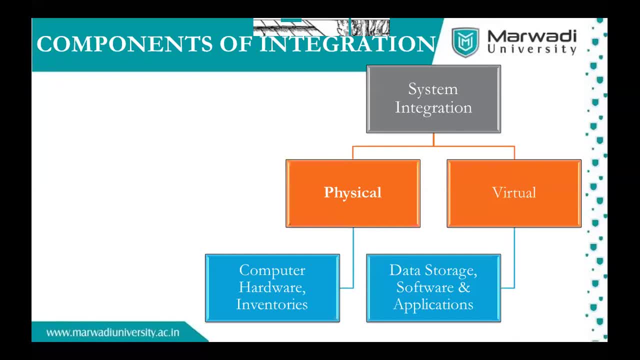 We have to look after the physical and virtual. There are two aspects: will be there for the integration in physical. most of the hardware, computer hardware and inventories will be there, And if you see the virtual, you have to talk about the data storage software, utilization of software. 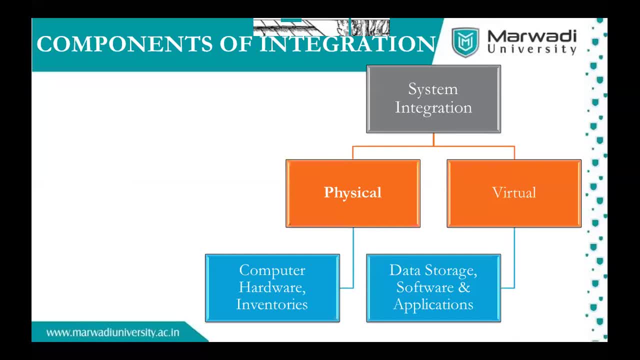 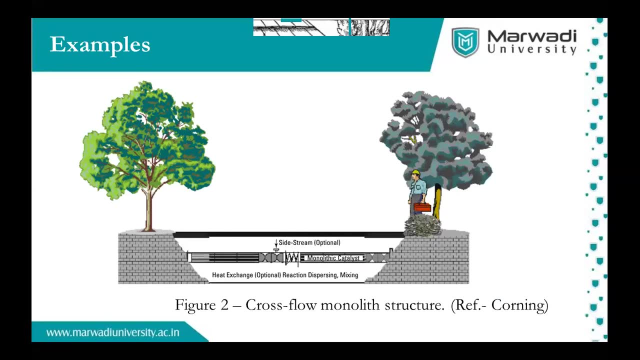 You have to use the software to integrate the process With this. yeah, the integration of process. Let's say, we are going to show you some examples only because, if we'll discuss this, this may take a lot of time and we are shortage of time. 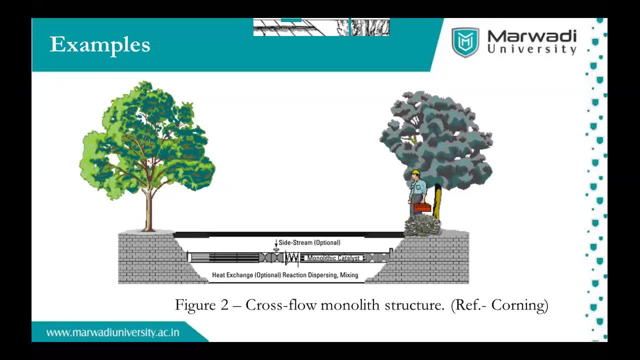 So this is one example which covered from the calling industry Where they are working. they worked on a monolithic reactor and they just tried to show you that monolith reactor. These are reactor where we are having a low pressure, low pressure drops. They can provide which kind of reaction system, reaction mechanism you are, you have. but if 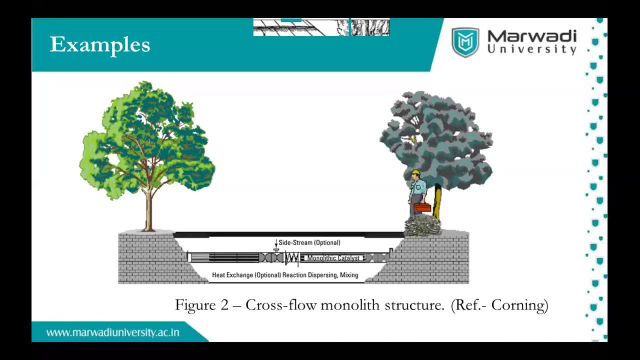 you can combine that monolithic reactor with different kind of, let's say, reactors and some heat and momentum and mass Aspects, what it can be done. So let's say a pictorial view on the right side, If you are able to see that one tree. 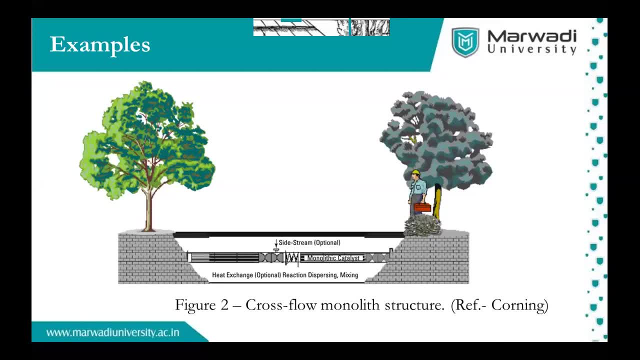 Which is, let's say, it is not having any components. Let's say: but when you started with this on the left side, you will be able to see that, the green tree. So let's say, it is like that When you are going for any pi, you are going to increase the efficiency of the system. 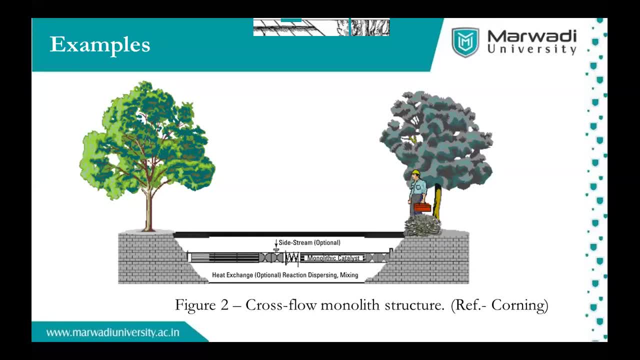 Okay, So as far as The picture is concerned, we can have different kind of interpretation. That is my own interpretation, which I thought to share with you. Okay, the next one. you can go through the website of Corning for different. 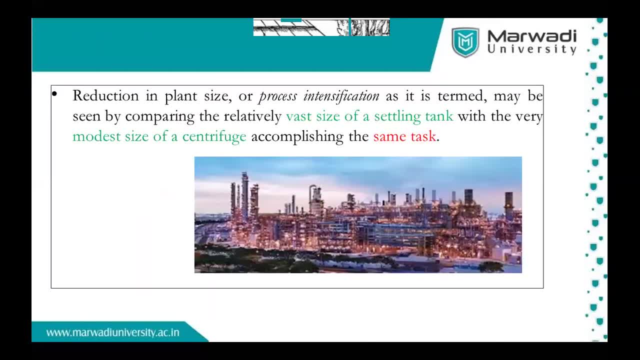 Yeah, methods. Next example, sir. Yeah, I will just, I will just try to, in short time, I will just try to show you that if we want to reduce the size of plant, what we have to do, There are different parameters We can have, let's say, in the figure, 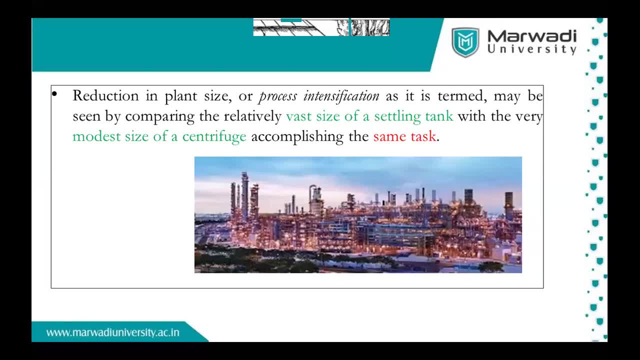 Which we have kept. on this slide you will be able to see that different columns, Those are standing in front of you along with piping right. So what is our need right now? We don't have these, these many parameters and this many resources. 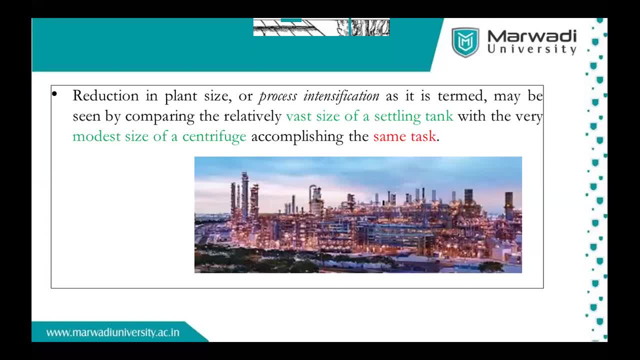 What we have to do. We have to combine all these things to reduce lot of utilities. It may cover n number of parameters, right, So it may. it will start from your basic Physics or mathematics to the technology aspects, Right, Yeah, next one, sir. 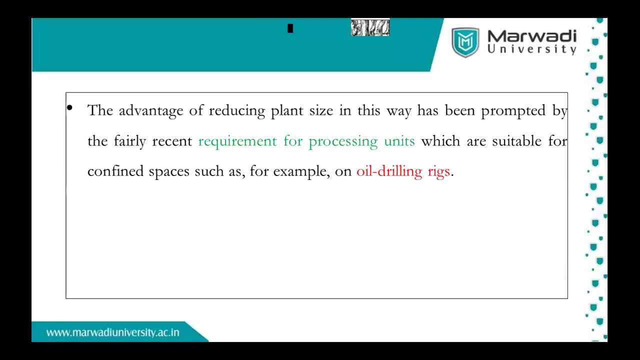 Yes, So this is one example. Yeah, Yeah, please, please, please, proceed, Yeah, continue, sir, Continue, continue, Yeah. So, as I had discussed in the last slide that we have to reduce the size of reactor, You have to check its connections, right? 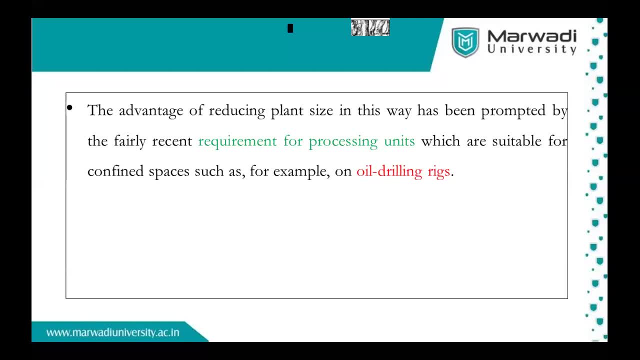 So one of the example which we thought to discuss with you was oil drilling rigs. So when we will have a next, let's say, a webinar, we'll try to discuss this in detail. The next one, sir, Next slide, please. 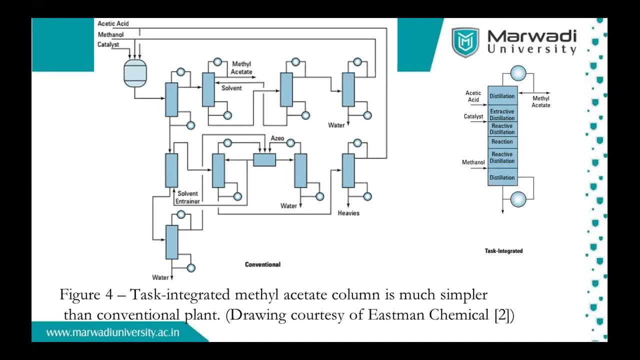 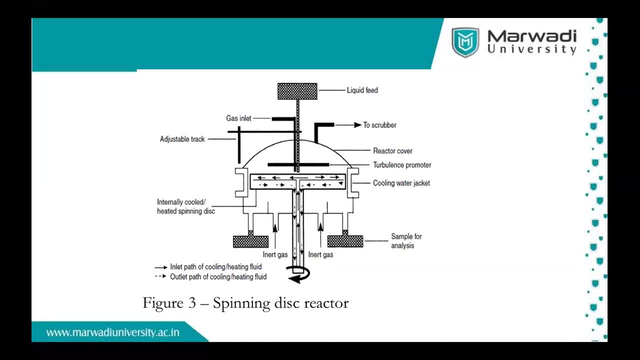 Spinning this reactor. It is also one of the yeah, let's, let us go for this. This is very, very important. This is given by Eastman. Yes, Spinning, sir, spinning. We will try to discuss in the next webinar. 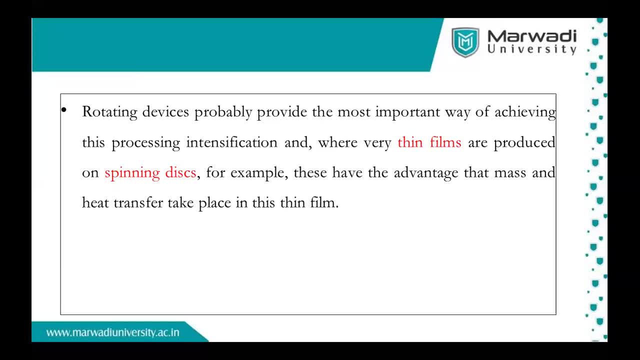 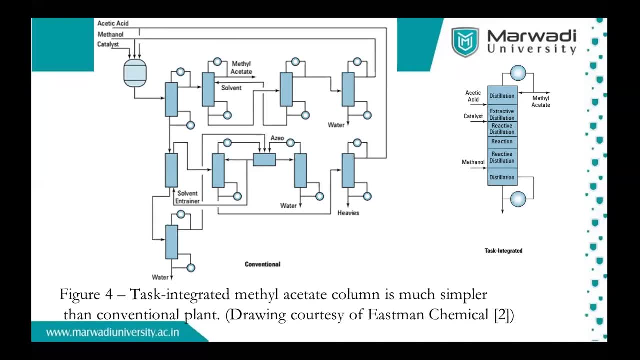 Whenever we will have a time to discuss this spinning So we'll go for the. yeah, this is from Eastman Chemistries Chemical. interested students in interested participant can go to the website of Eastman chemicals. See, on the, let's say, left side, you will be able to see that the PID which has shown 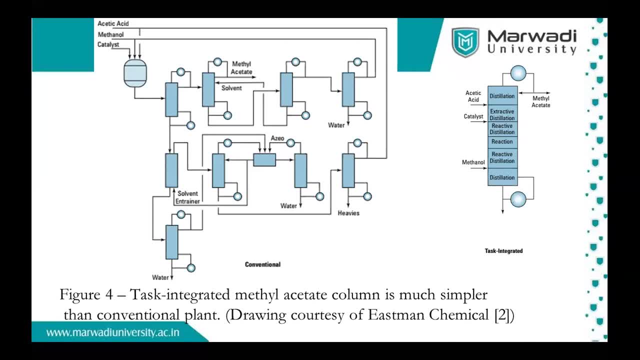 the different kind of parameters, how the reactors are connected and how we are getting the product. But what happens in the task integrated, which is on your extreme right side, that all these unit operation, unit processes are combined in a single reactor and your system. 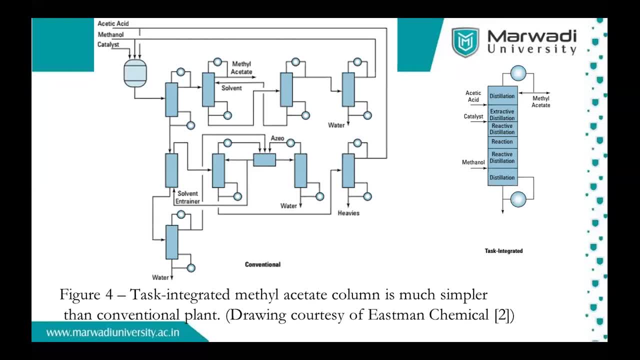 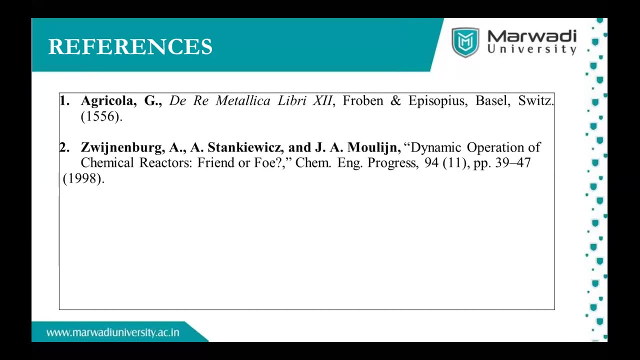 Now it is ready to work for right. So this is what the integration of different processes is. Okay, Yeah, Next one: Yeah, these are the references which we have cited in today's discussion, And thank you very much Everyone. 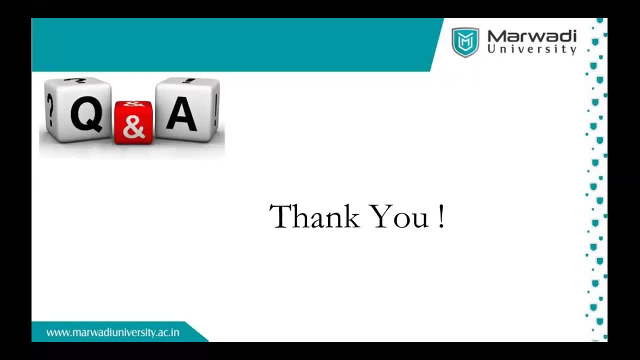 Those who are here to on their interest, to study about or to discussed about Process intensification. Please note that this is very vast subject. If Dr Manish agree with me that this is not being covered within an hour or so, it will required. 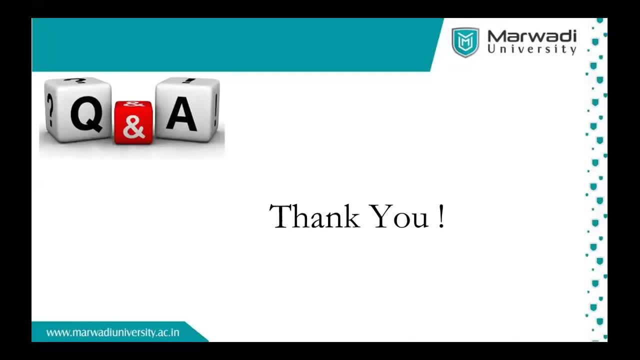 so much time to understand the different aspects, But our aim is to highlight the different processes which can be intensified with the help of this technique. So, as an initiative taken by the Marwadi University, We thought to share Our expertise. Okay, and if you are having any queries, you can raise your hand. 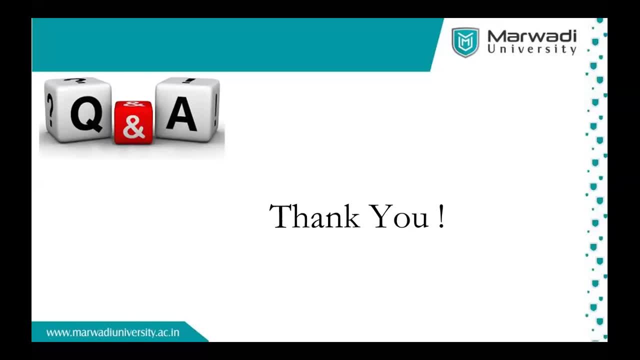 And if anyone wants to give you a suggestions also, it is always welcome. Apart from this, I feel sometime before we had. Yeah, we have one of the participant, Abhijit Kulkarni. Abhijit, are you there? 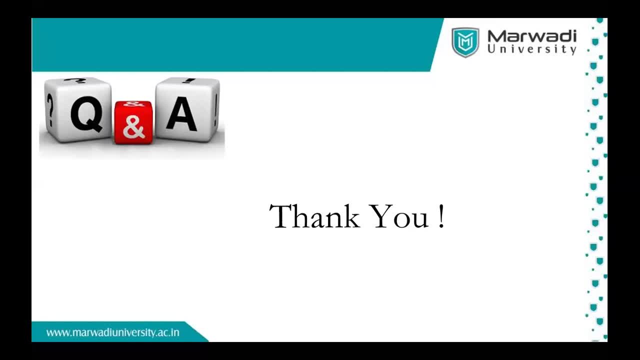 Abhijit: Yeah, Yeah, Yeah. Good afternoon, Abhijit. Actually, I just want to yeah, Yeah, I just want to Yeah, Abhijit is one of the entrepreneur. I know him as he worked with me. 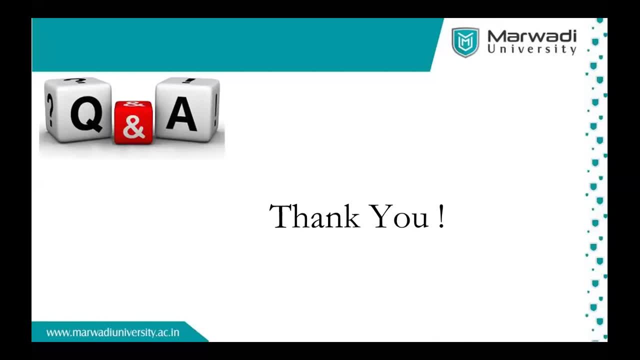 He's working on the same area itself. Abhijit, do you want to share some views based on it within a minute or so? Sure, Sure, Of course, Means. I was about to raise my hand, So, before my sharing experience, I would like to ask Mr. 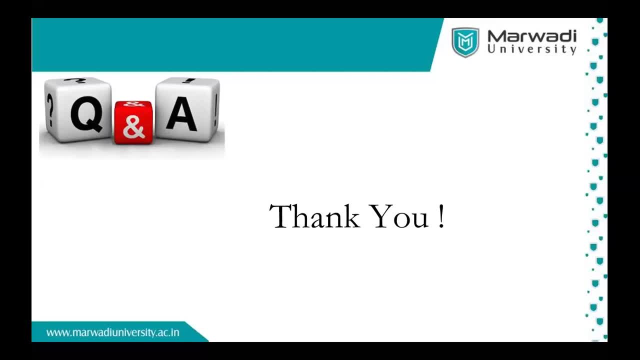 Manish sir actually request. So can you just elaborate more about the software integration over this PI? Software integration means, sir, if you are using ASPEN and HiC And if you are able to do the proper process, so it will give the accurate design. 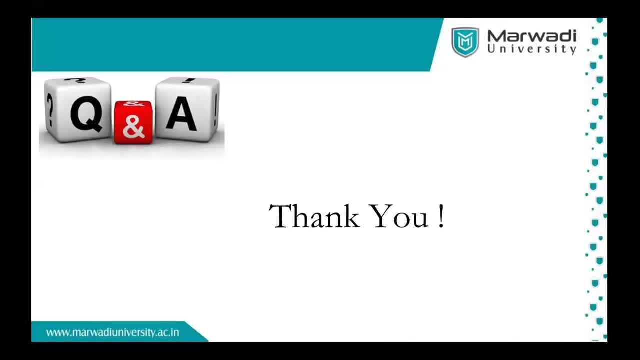 If you, if you take, for example, heat exchanger, and if you apply the ASPEN and if you are able to get the proper design of the heat exchanger so you can say you are utilizing the software and you are the accuracy, accuracy towards hundred. 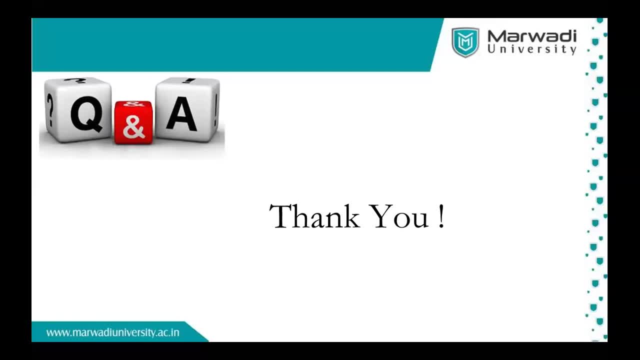 Yeah, But if you do the trial and error, if you are not able to design the properly, then your approach will not be towards hundred hundred percent. So you have to utilize the process, software process, to make the process is more and more accurate. 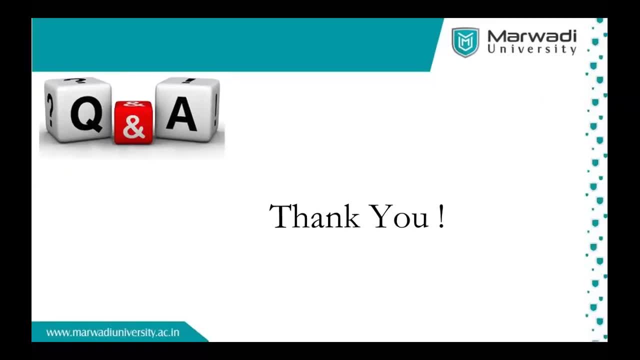 Okay, Thank you sir. So, Ritesh, Yeah, so basically, as the sir has already told, that, they have scaled up their reaction in the while they were working in the industry. So basically, we also deals with the same kind of process and same kind of industry and we have almost converted so many batch of batch reactors or batch data to the continuous 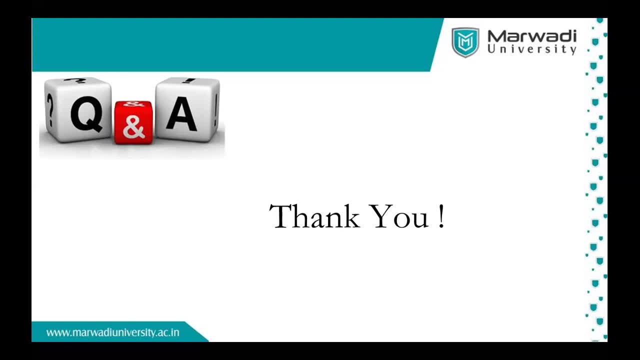 So reactions such as John's, oxidation and epoxidation, So many reactions- We have also converted to the continuous scale up. So, basically, what we deal with, we also deal with the process intensification and currently we are dealing with the micro reactors. Yeah, yeah. 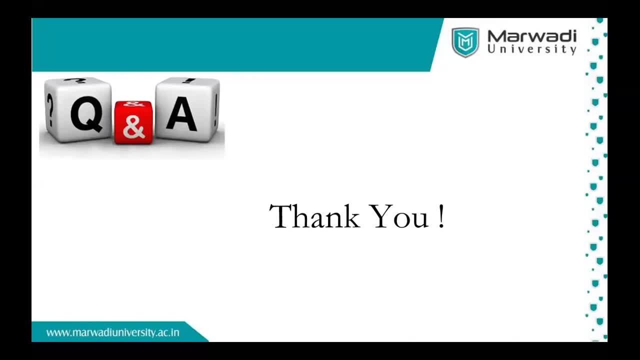 In addition to this, I just want to inform our viewers and participants: Abhijit has worked with Corning, If I'm not wrong. right, Abhijit? Yes, Yes, you work with Corning. Corning technology, Yep. 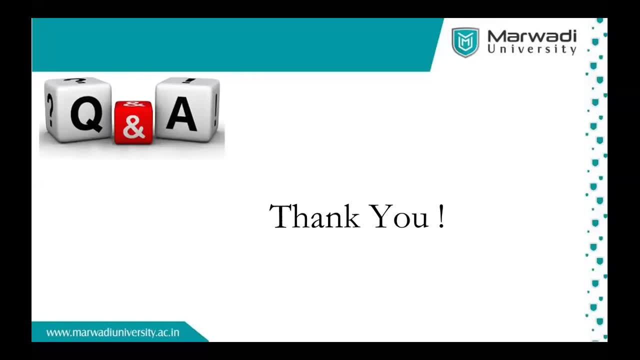 Continue, Abhijit. Yes, So my startup name is Florex and we are also working on the distillation. So we have received a government grant for the continuous intensified distillation. So we are currently working on it on the similar basis so that, as sir was seeing, integration of all the technology. 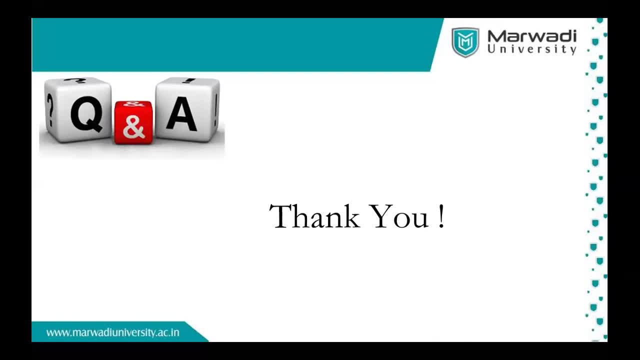 So currently we have our demo and we have our equipment for the micro reactor- So we are also working- or for the different processes like distillation and extraction- Great So, so that we can integrate all the process technology. So from it's like start to end, everything like process downstreaming and process reaction. 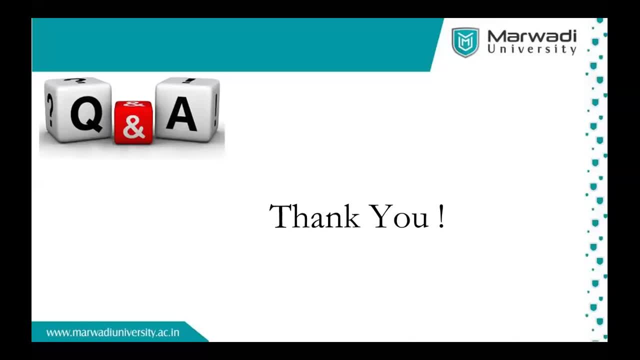 Yeah, right, Fine, Fine, Yeah, Thank you very much, Abhijit, sharing your views, As he is One of the, let's say, and he's of your age. Only those were participants, Let's say. I want to keep your attention like this. 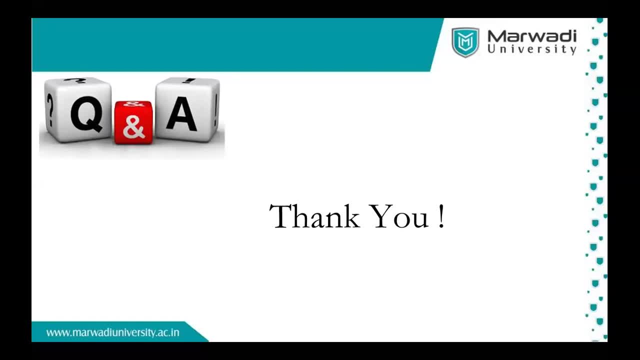 He is one of the youngest entrepreneur with whom I personally know and who did his growth. Actually, he is from my friend circle when I was doing a PhD, and this is a group of four or five entrepreneurs- Those who are working from last four to five years- and you cannot believe this, that these guys 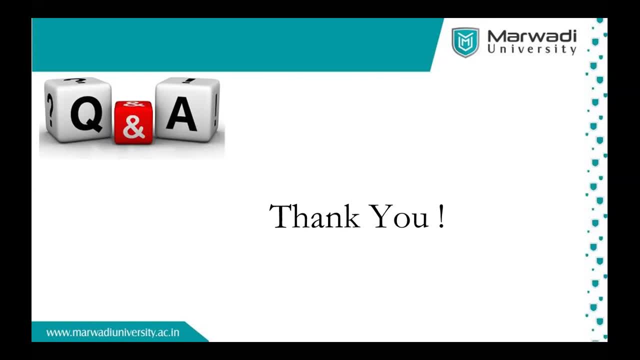 Are very fabulous. They have working for government grants in, let's say, at the age of 25 and 26.. These guys have grabbed so many funds right, Abhijit. Yes, Yes, sir, And thanks. Thanks a lot for your this great initiative by the Marwad University. 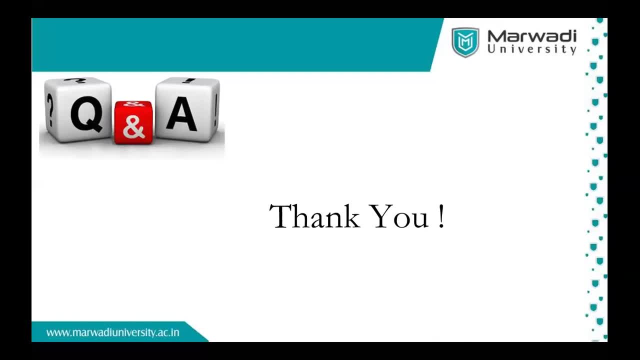 It's really helpful during this lockdown period so that we can share thoughts with each other. Even I don't know the participant. mostly I feel they will be student- Yes, but I can suggest them. They are free to call anytime for if they have any queries. 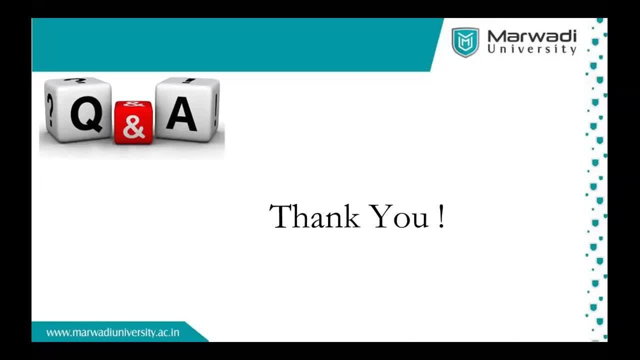 Even I would like to interact with you and even with your other faculty, with the Marwad University. Definitely, Abhijit, I will. I will plan one, one session, Let's say for one hour or so, with the other students, like this webinar. 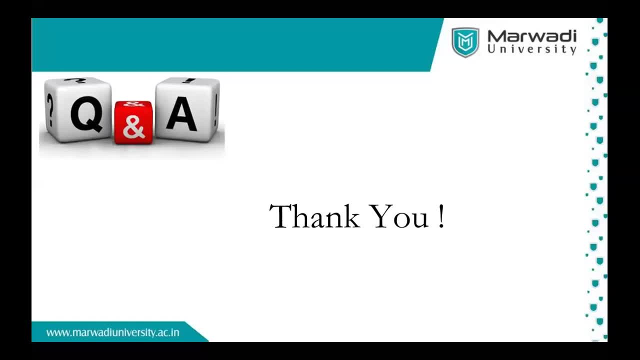 So we will have a interactive session with you like interview, right? I will communicate him for sure. Sure, Okay, Yeah, Thank you. Sure, Thank you, Abhijit. Yeah, Yes, sir, Thanks a lot Yeah. 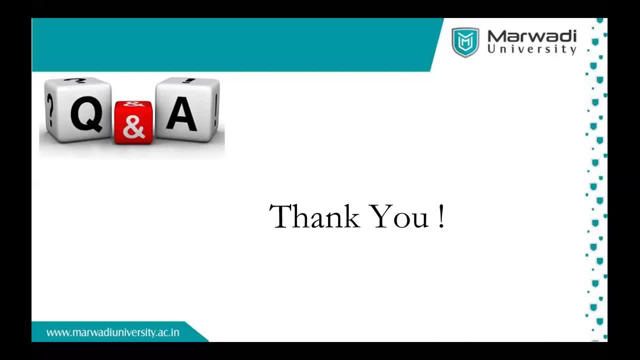 Thank you, Abhijit. If someone, if anyone, is having any queries, doubts, they can write to us. if you want to discuss right now, please raise your hand if you want. Otherwise, let's, we can stop here. Okay, I feel that this is. I take this opportunity to say thanks to everyone. 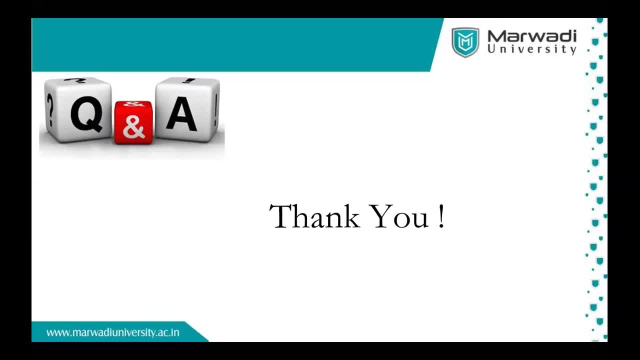 Thanks, Thanks to Professor Manish Khodve to share his expertise along with me, to the students as well, as we are having some participant from from different states, Also those who are participating in today's webinar, So I feel this is a kind of, let's say, little donation from our side. 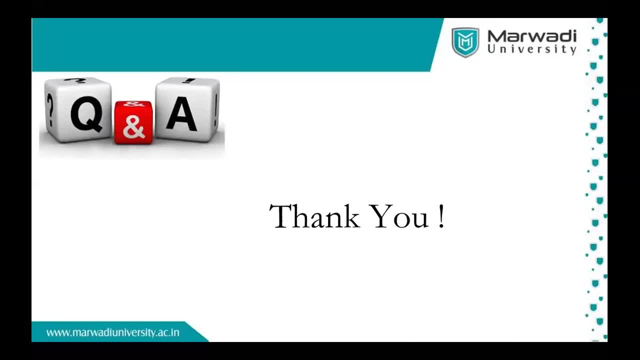 Let's say, sharing our knowledge, which we are having. still, I just want to add to this: We are also learning right? So as we will share our thoughts with others, we will be able to nourish ourselves. Okay, so stay at home. 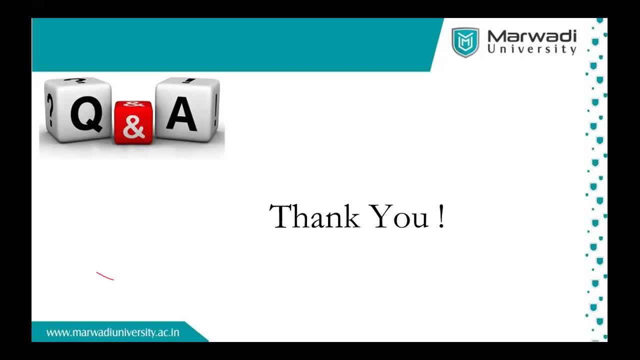 Stay safe and keep learning. Thank you everyone for joining to us. and one more request: I just want to have the email ID of all you guys who are present right now, so you can type your email ID's. Okay, proper email ID's. 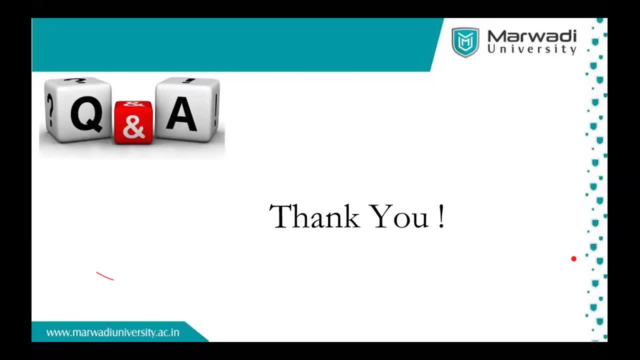 Okay, proper, your email ID's Please try to put in the chat box So I can make the further announcements either. in terms of certificates Also, we are proceeding for this, So in due course of time we will communicate with you. 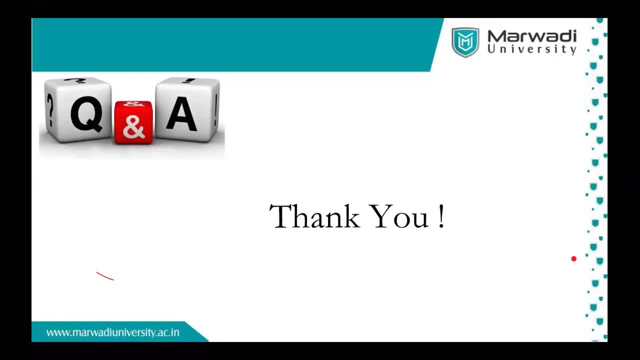 So all of you are requested to put your email ID's in chat box. Yeah, Thank you very much. Thank you, Praveen sir. Yeah, one of the faculty who joined us from SDGS, Nanded Praveen Sonarkar, Dr Praveen Sonarkar. 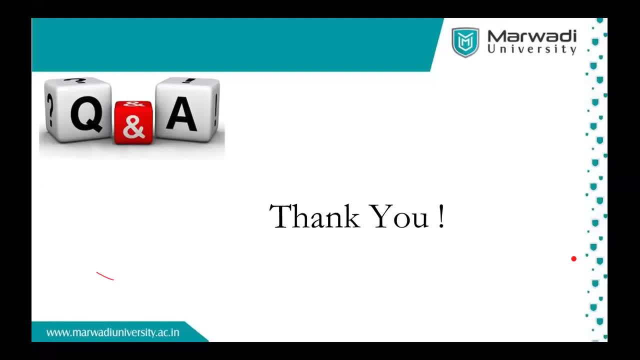 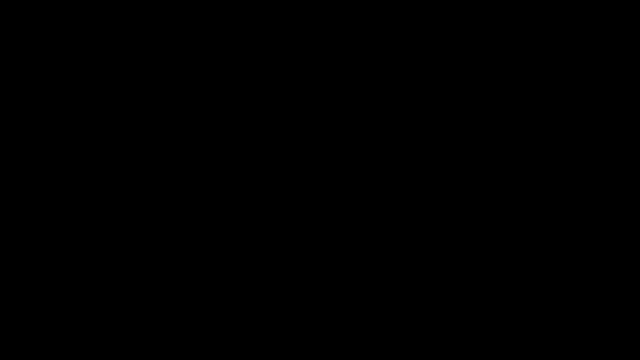 Thank you, everyone joining for this. Thank you, Yeah, Hello Sir. Hello, Yes, Sir, there is no chat box in this Chat box. I don't know, Sir. we will message Ditesh. sir, We will do that. 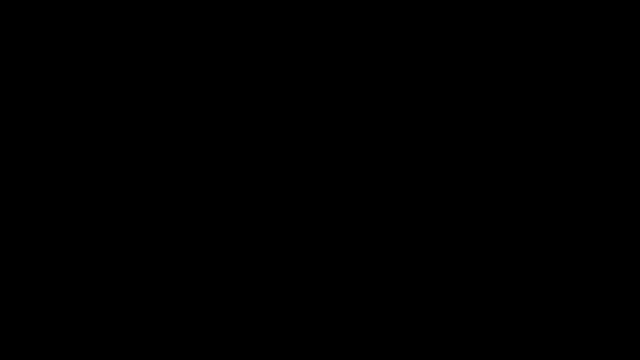 Yeah, We will message him. The host is getting a lot of messages, right? Okay, sir. We have messaged you in private, sir, Your email ID: No, no, no, We haven't seen the zoom chat box. 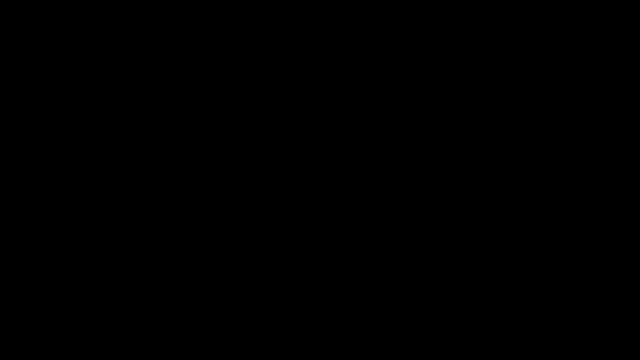 It must be coming. It's coming. Please check it. Please check it now, Sir. it's coming. I have sent it. I sent it, sir, I want. I want this in chat box only so I can have that proof. okay. 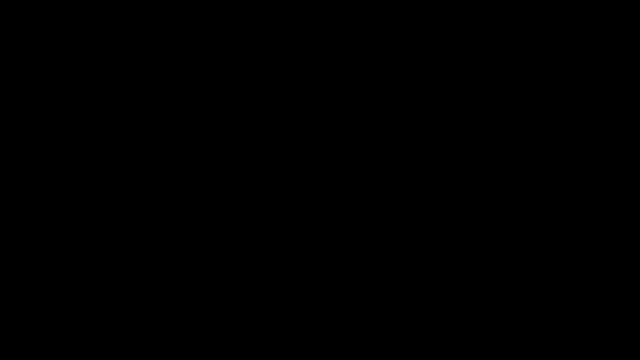 Please do not message me, Sir. Do not message me on my phone. You are requested to put your email ID's. Okay, Sir, it's not coming in this, It's only yours in personal. Dr Ditesh Parker is hosting it. 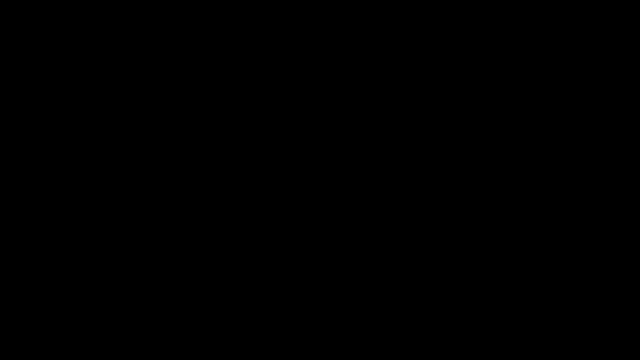 So text it and post it. No, no, it's not happening. Everyone, Everyone, Everyone, do it. Son, do it in it. It's happening. Yeah, yeah, Please, please, Please, explore it, Please explore it. 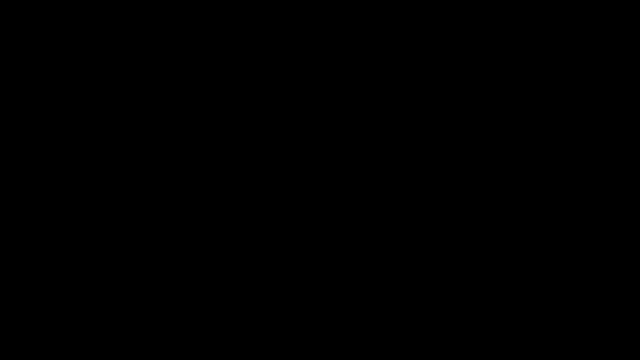 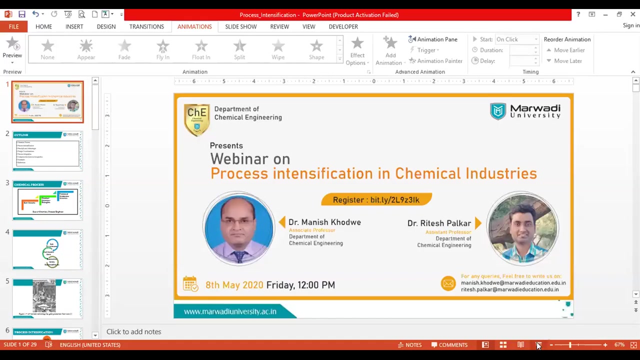 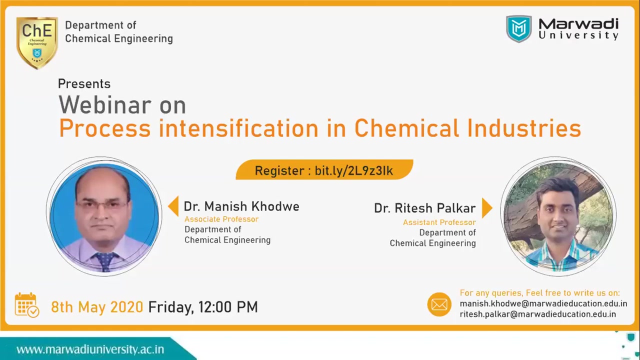 Ah, yes, sir, It's coming Letter. My email ID is coming. Thank you for joining all of you. Thank you, sir, Sir, sir, Yes, sir, Do you want to continue or leave For a minute or so?